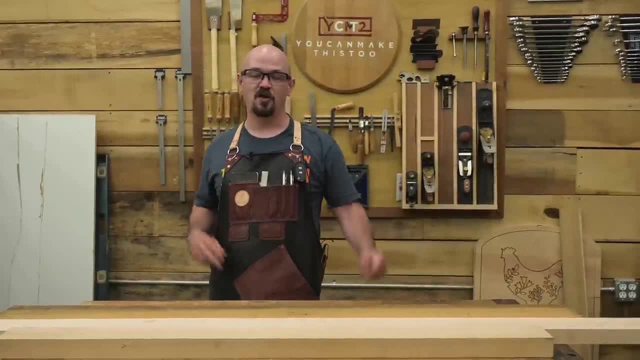 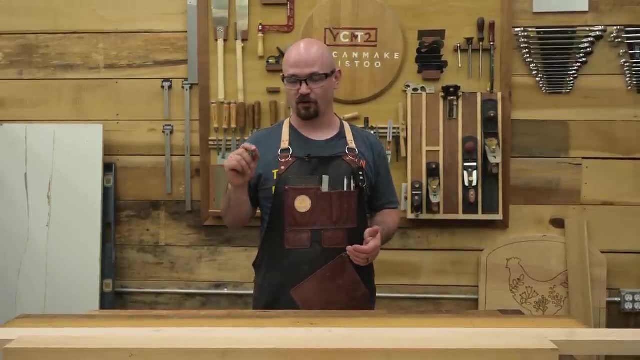 boxes, or you just don't know. You just want to build something. That's cool. I have a recommendation for the second best, then, which I guess would actually be your best, so it's still the best. Whatever A table, I think it checks all the boxes for a great beginner or even first project. I. 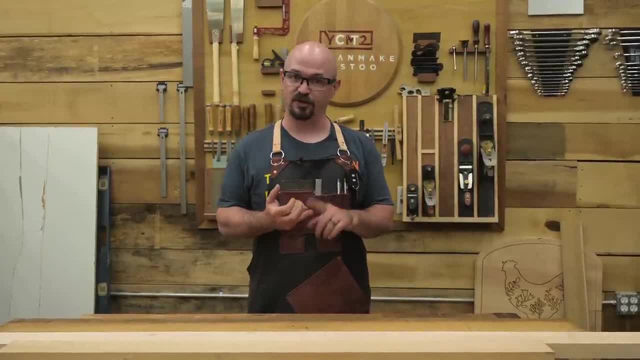 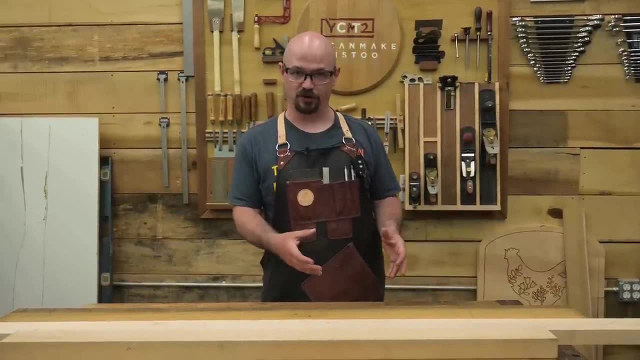 think a great beginner project should be something that's very approachable, something that's going to be useful for most people who can't use a table. that scales The principles we're going to use and how we build this you can use to build a side table, like we're going to do, or a sofa table. 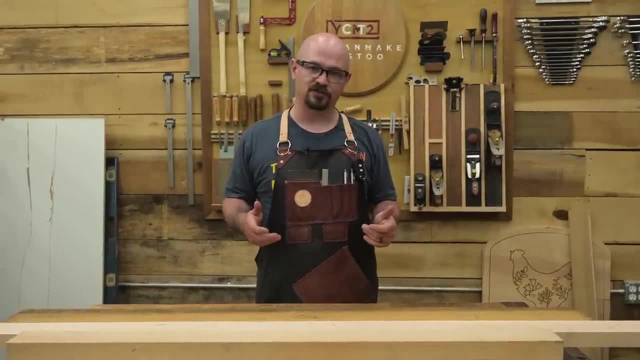 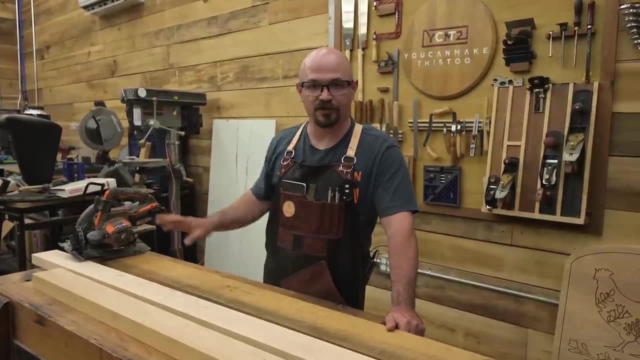 a dining table. Principles all apply and get to exercise a lot of the fundamentals. It should also be something you can build with a very basic tool set. I've always sworn I'm never going to do this, but leaving all my machines alone, and I'm only going to build this with some really 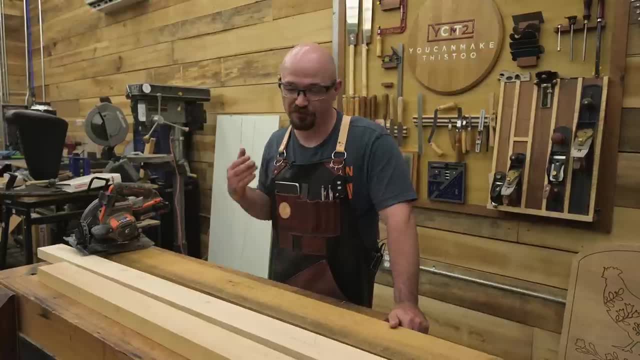 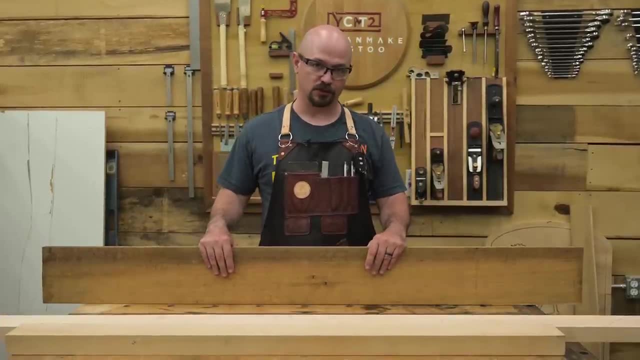 really common tools that you probably have can get very affordably or a very good chance you can borrow from a friend because they're common. First thing we're going to do- I'm just using some scrap here- is I need to do a glue up to make my top, which is a panel, glue up. 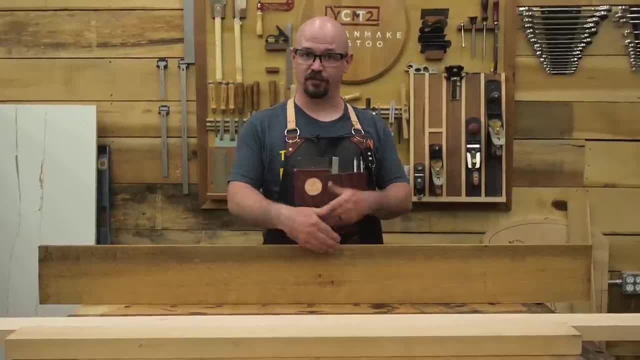 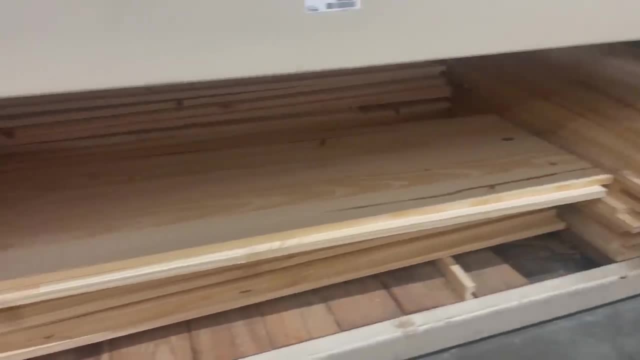 very common in woodworking. If, for any reason, you're not set up, the nice thing is you can either buy a board wide enough or Home Depot and Lowe's in the more section- normally down low on the shelves- Both of them actually have pre-glued up panels of various sizes, so get the size that. 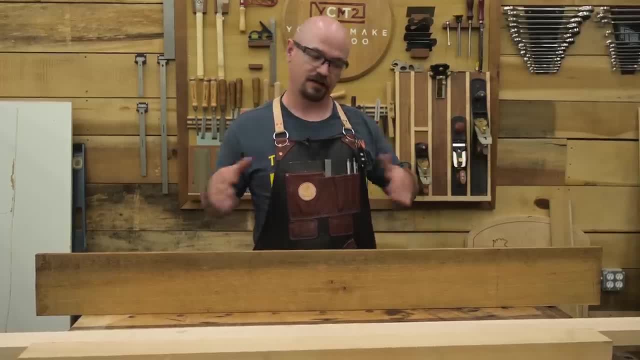 fits for you, or is it a little bit larger and then cut it down to the size you need? if you're not set up to do a panel, The table I need in my house- I'm going to be using a table that's. 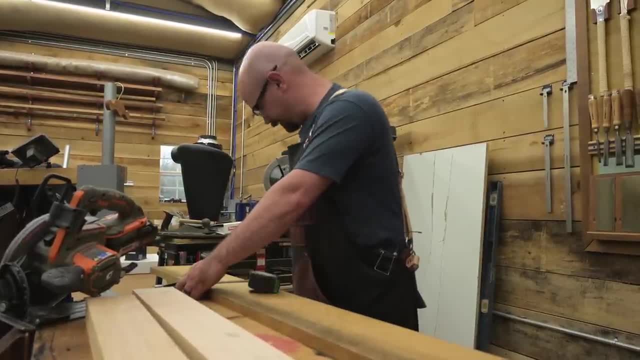 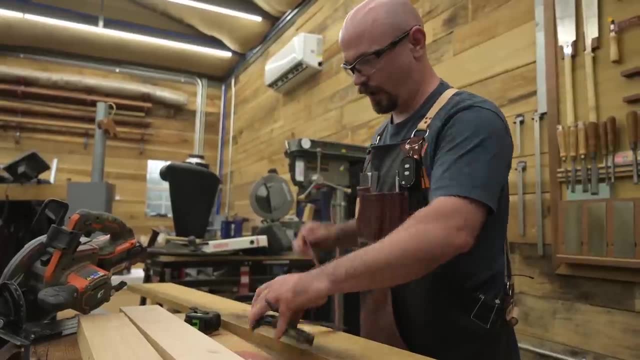 is a little triangular table to go in the corner by my back door because we've got dog collars and stuff and there's no good place for them. This top is going to happen to be white oak and then the legs are maple. This could all be pine, poplar, cedar. whatever you have, whatever you can get. 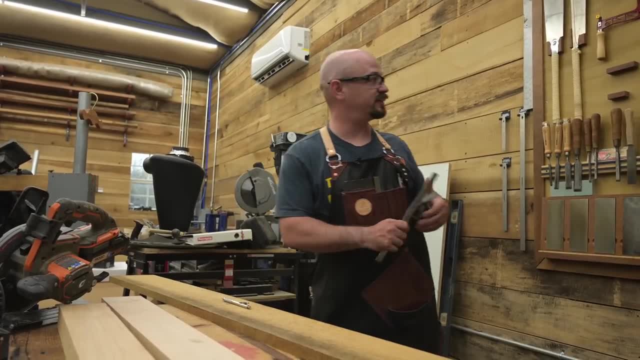 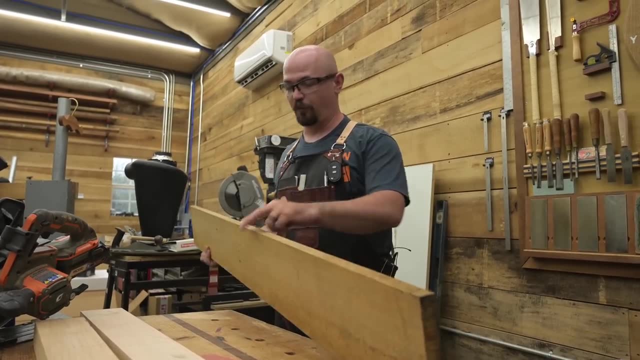 I do recommend, if you probably don't have milling machines to work with rough material, This is already surfaced on two sides. I've already machined it at some point for a project, so it's smooth on both sides. Go buy wood, that's already smooth on two sides. 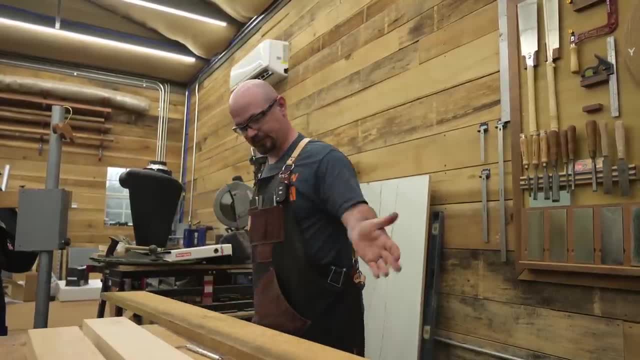 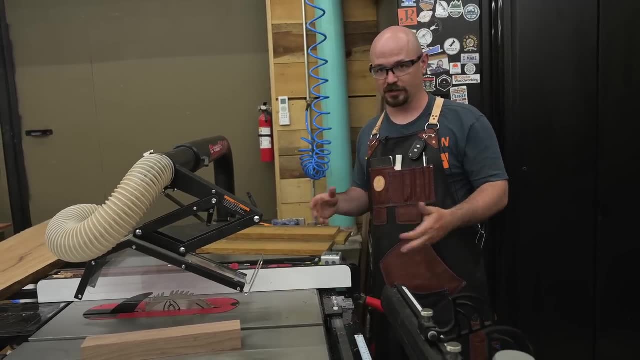 Because otherwise you've got to go through the whole milling process. First thing I'm going to do is just cut this down closer to the sizes I need. If I had a little contractor tabletop table saw I would use that. I don't. All I have is this. 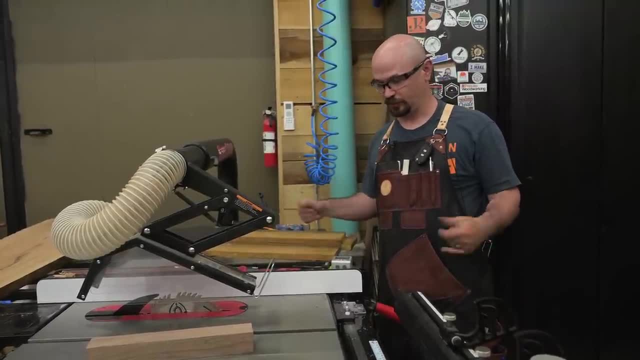 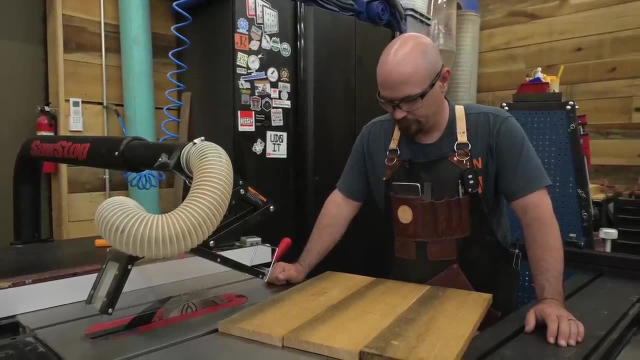 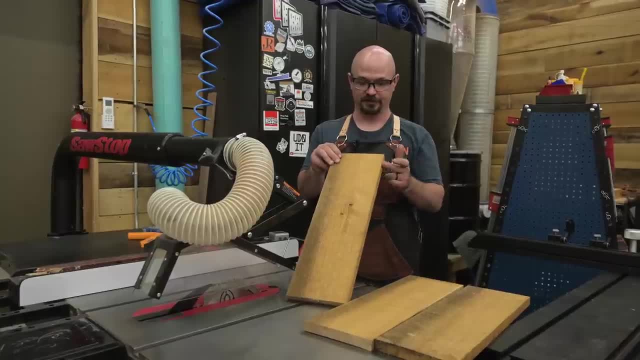 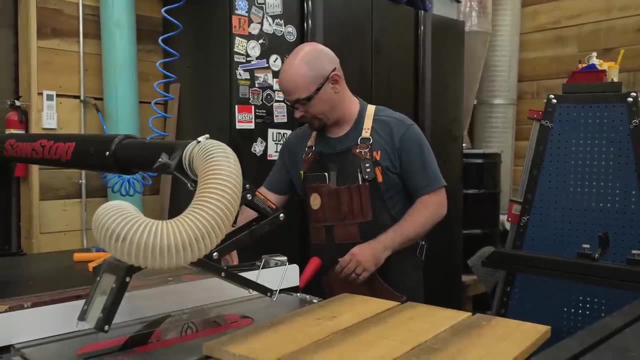 And they're really nice and square to the face. So this is the face, this is the edge. You can skip this also, especially if they're straight- Mine's not. So if it's not, a hand plane would be another option. but you need to straighten them up And that's what we're going to do here. 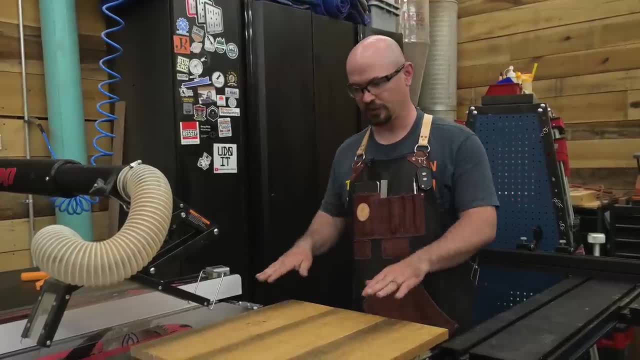 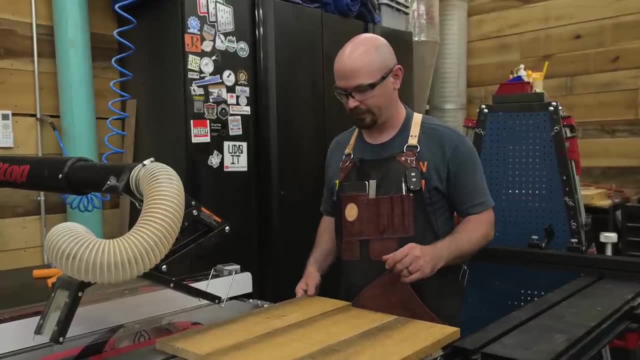 at the table saw. There is a little bit of a trick to jointing at the table saw when we're going to do a glue up. My blade is very, very close to 90, but not exactly. The more off the more obvious it is. So what I'm going to do is mark on the end of my board which side is. 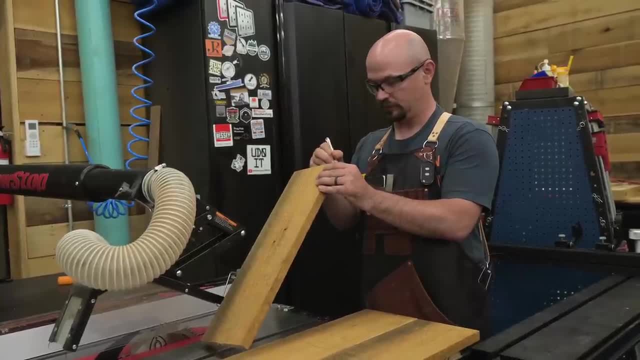 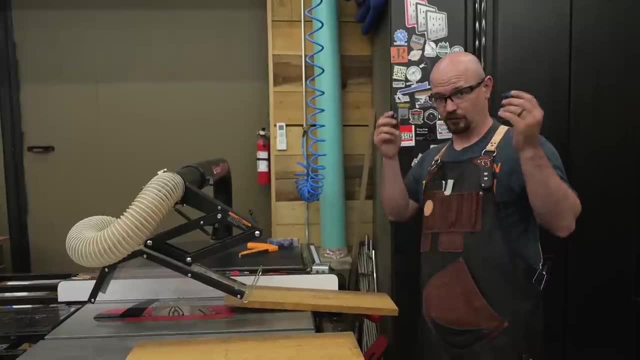 and against the blade. So I'm going to make a little notchy-do. So I've got a little indicator. After I do all my cuts, I'll show you how I line these up. after And when you're using machines and power tools, remember your PPE eyes and ears. 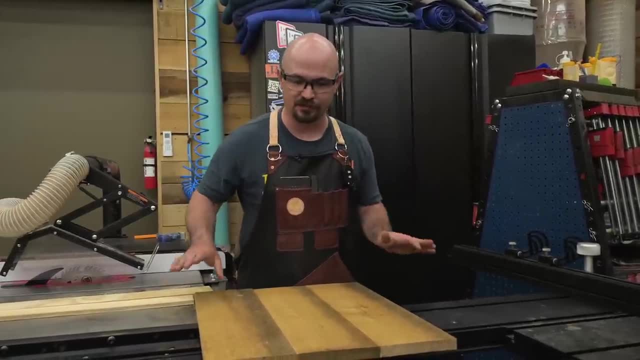 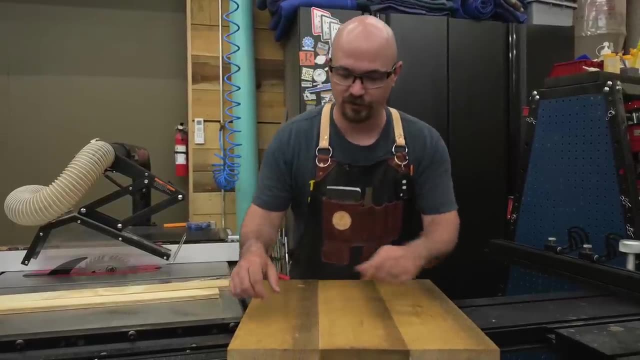 Now this board happened to get cut on the outside edge. This one didn't Doesn't matter at this point, Because the inside is where we're gluing, not the outsides. We have nice clean wood on the inside and out. Now, as far as the orientation, you'll see that they alternate. This cancels out. 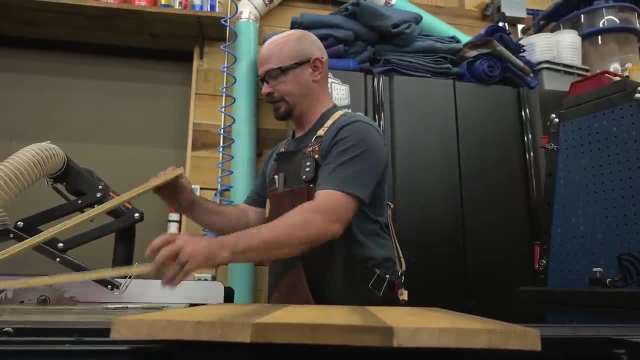 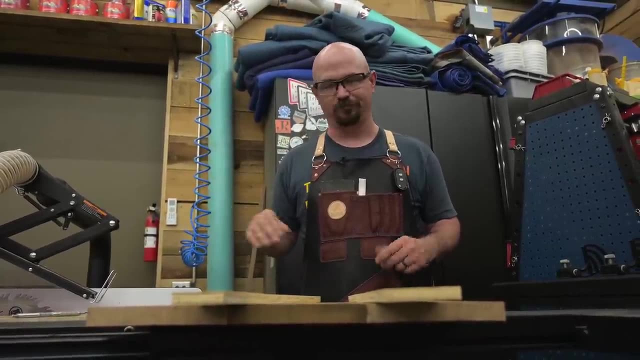 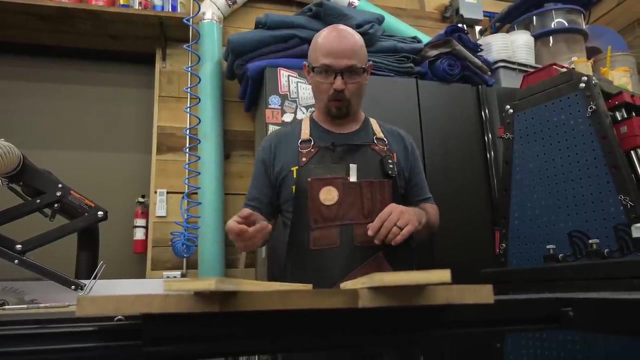 any error in the blade deviating from 90. I can show you, Because you kind of have three options here: Either your blade is somehow perfectly set up, which it's probably never going to be, or you cancel out your error by aligning things correctly, or you double your error making it. 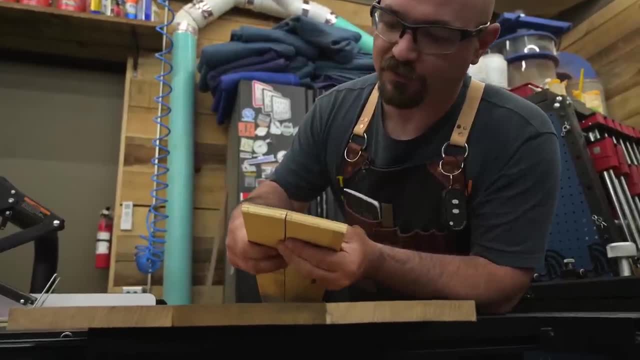 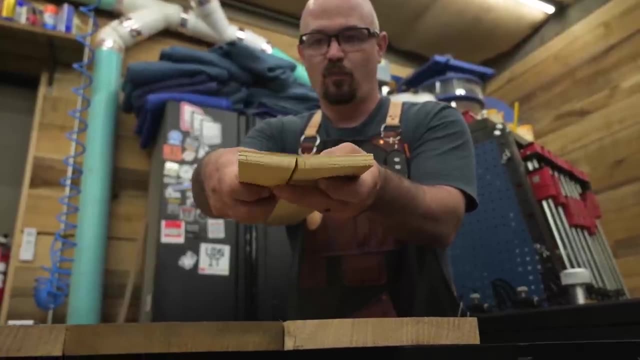 so you, either it's perfect or worse. And notice here, if I line them up, the same instead of alternating, and what I did is I just cut these at a more severe angle so they show up. See how, instead of flat, it's like whoa. that's not cool at all. But if I come over here and do the 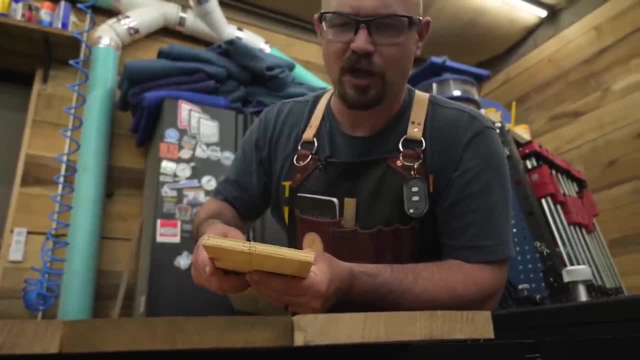 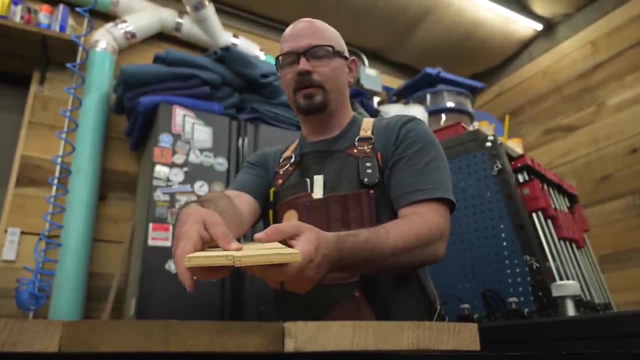 alternate. see, there, I forget my geometry Complementary. I think that's called complementary angles, And now it's flat on top, So it canceled out. Now, obviously you don't want to do this willy-nilly and not care what your blade angle is, Because if I try to glue this and it's too. 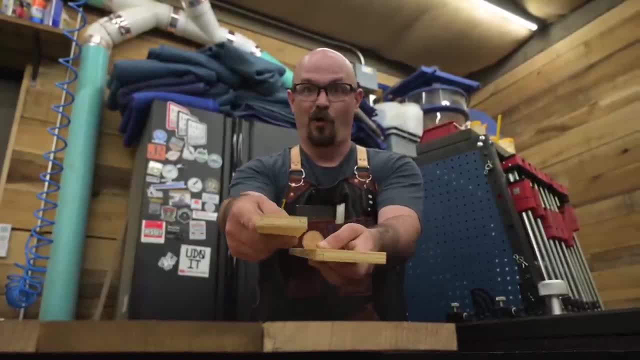 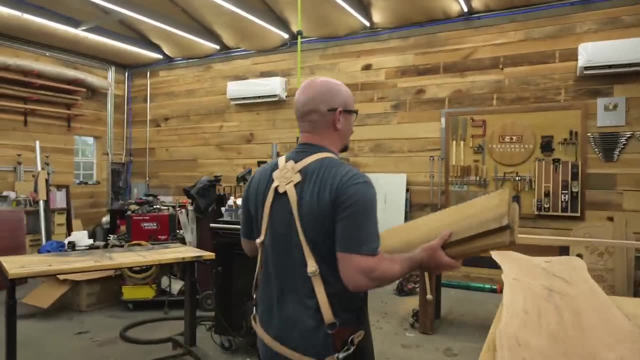 severe. the clamps are actually going to make them want to. you know, slide apart. So you do want to be close to 90. Especially if you're beginning, you probably never want to glue up more than one edge at a time. The amount of error you see there might not even be noticeable, But if 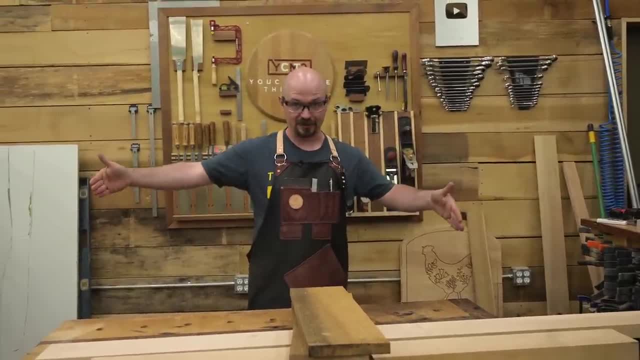 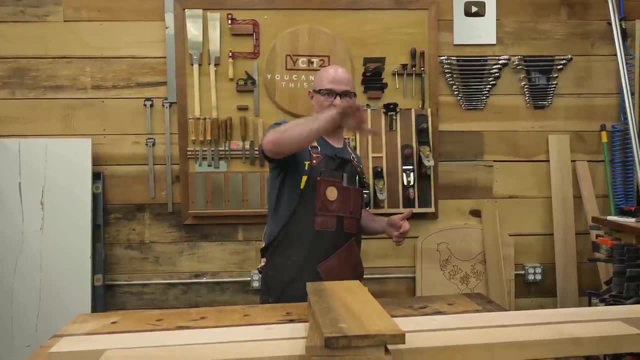 you're doing a larger panel where you have four, five, six, seven, eight glue lines and you're kind of willy-nilly each time. you know that error magnifies and magnifies and becomes more visible. Now I'm using a combination blade in my table saw. 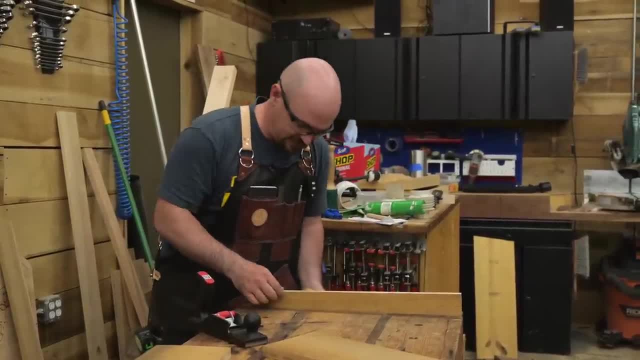 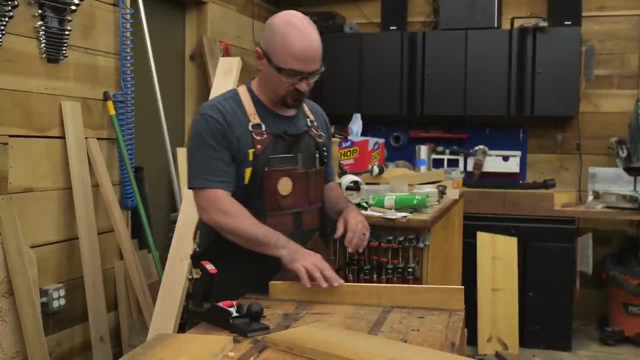 And it's a little old, So it doesn't give me the absolute best edge. There's some tooth marks, And what will help minimize that is cutting really slow. I was cutting a little fast And so I have all these ridges which come up with a fine glue joint. This would still come together fine as is. 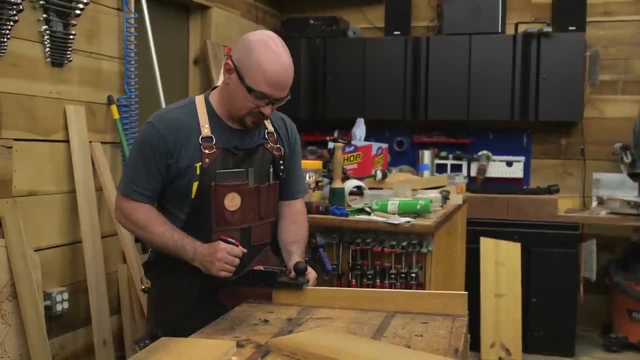 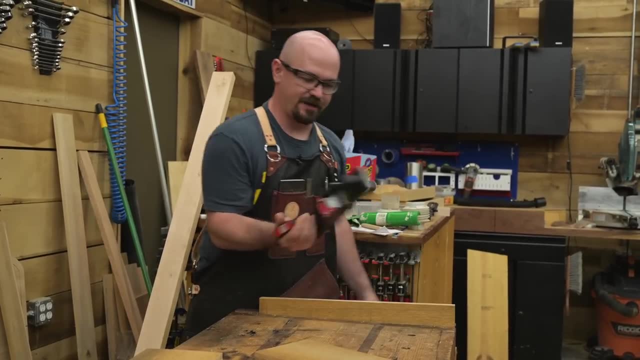 but I want it to be a little bit better And I do have hand planes And I feel like hand planes are pretty common. So I'm just going to do a few swipes just to smooth this out some. I have a video out. 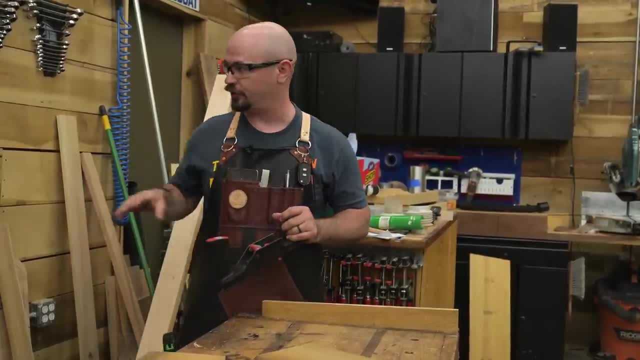 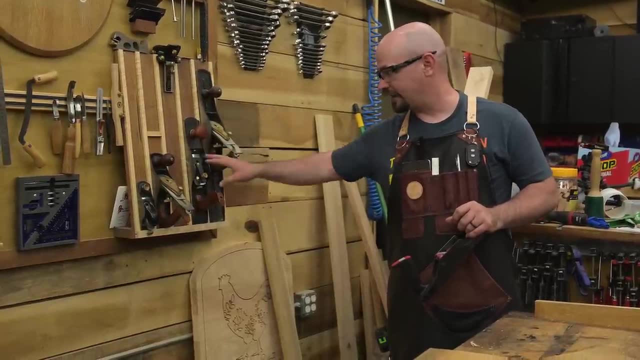 about these specific planes. These are great for beginners because everything that intimidates you about normal traditional hand planes like I have over here, you know: having to have a sharpening setup, learning how to sharpen, how to set up the plane, dial it in and then use it. that all goes. 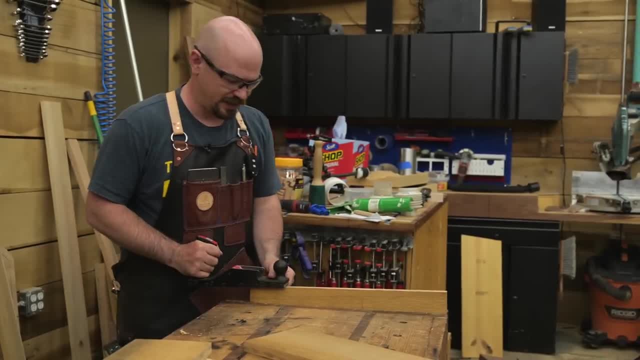 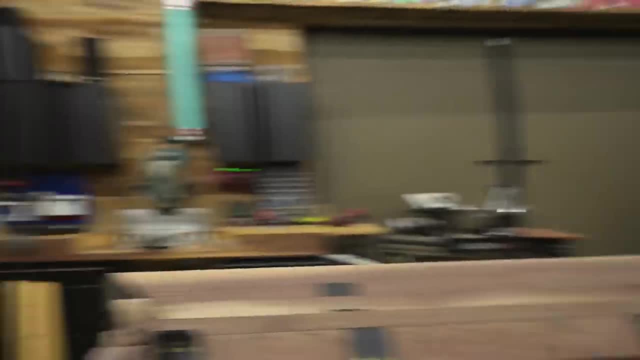 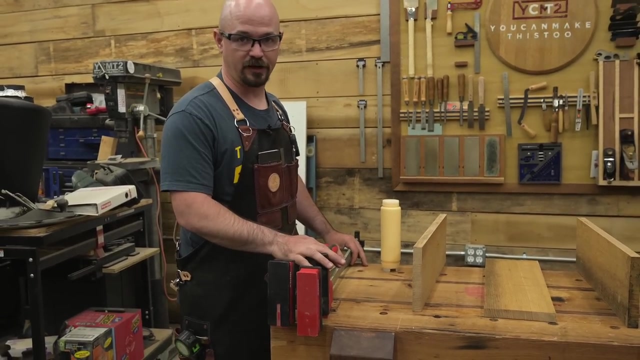 away. It's literally one little lever and the blade self registers and they're very affordable. So this hurts my heart. But in fairness to you, my beautiful parallel bar clamps are going to stay right here and I'm not going to use them. Glue- any PVA glue is fine for. 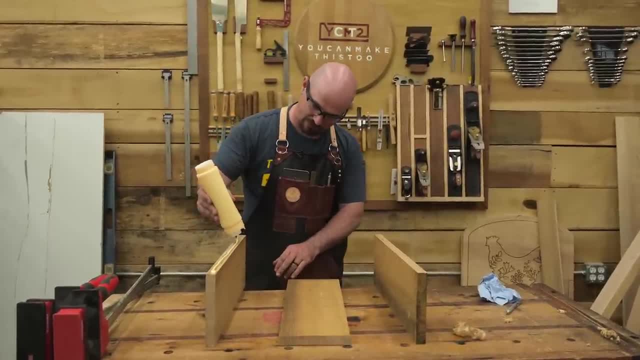 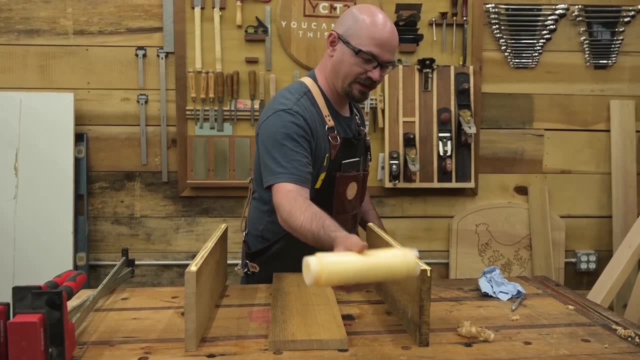 wood. This is Titebond II, and I just like these little upside-down condiment squeezers For the same reason. they're awesome. when they finally started putting ketchup in upside-down bottles, It's just there. That was honestly way more glue than I needed, And here's something I used to. 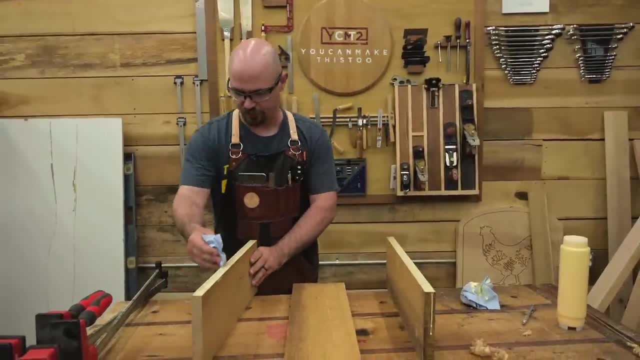 wonder: Can you glue just one, put glue on just one side, or do you need to put glue on both sides? Well, I've only put glue on one side for a long time and I've never had a glue joint fail. 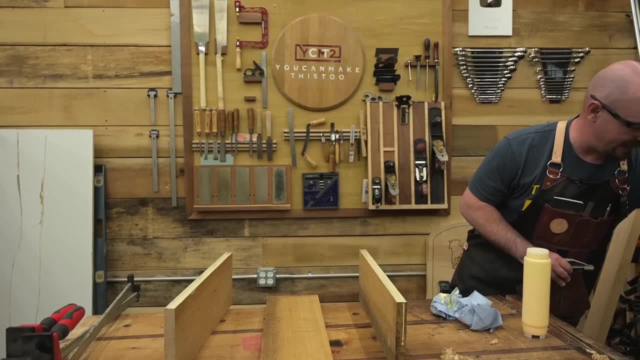 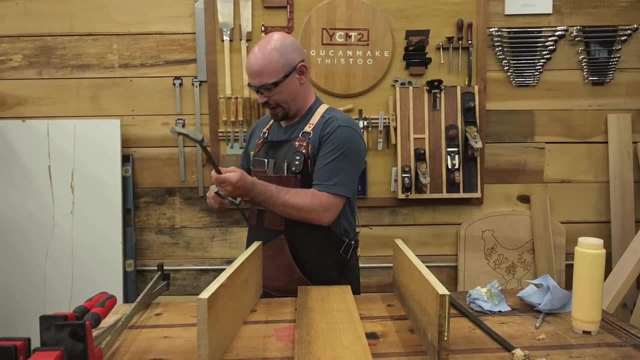 And the reason, besides my experience, that I felt fine with that is I was listening to a podcast with the CEO or president of, I want to say, Gorilla Glue, and he was asked that question: Hey, you're a glue expert, You make glue. 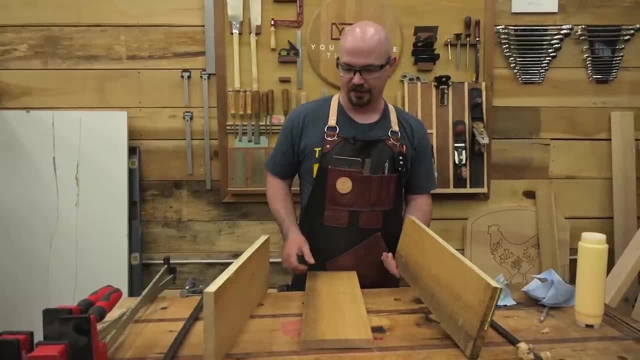 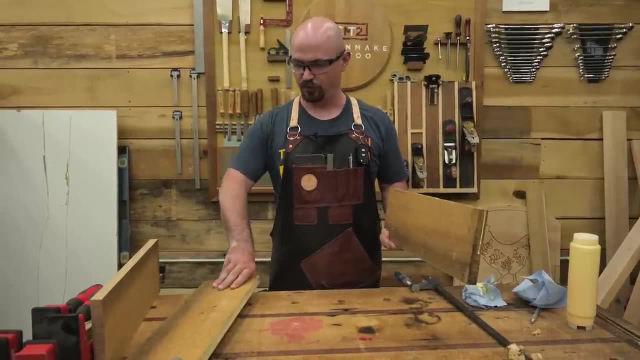 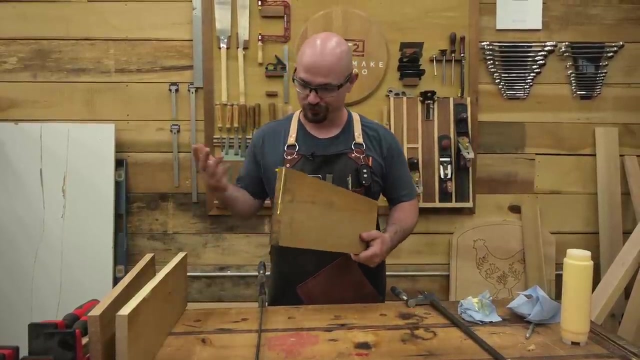 what do I need to do? Do I need to do both sides or one side? And he said: you only have to do one side. That's fine. But they do like people who do both sides more because they use more glue. So you sell more glue if people use more glue, So do with that what you will. So I'm going. to close this up for now. It's fun to be cooking the game, but I think it's exciting to see that you've done that And we'll be back with another lesson. See you in the next one. Bye-bye, Bye, Bye-bye. 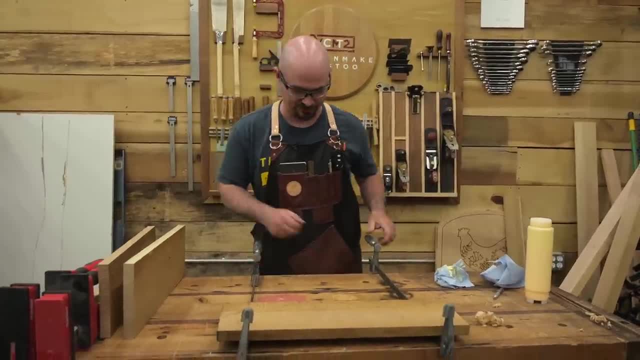 Bye-bye, Bye-bye, Bye-bye, Bye-bye, Bye-bye. with that what you will. So I'm just gonna use these F clamps because I don't have bar clamps anymore. Sold those a while ago when I built up my parallel. 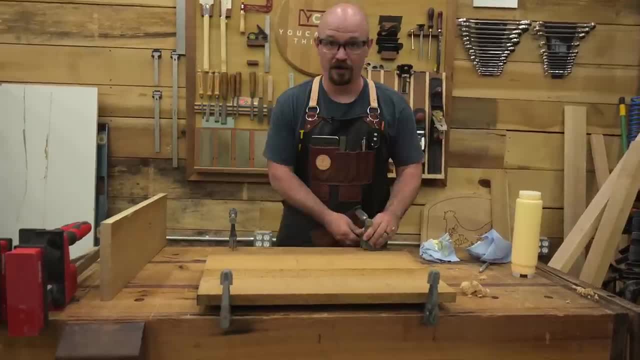 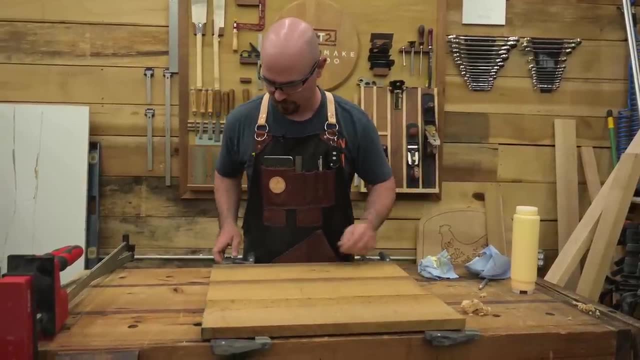 clamp collection. This is not at all what these clamps are for, but it's gonna work. That's the point. Use what you got. Alright, once I got these together, I'm just gonna give them a little shimmy. Really help work that glue in. You might be thinking. 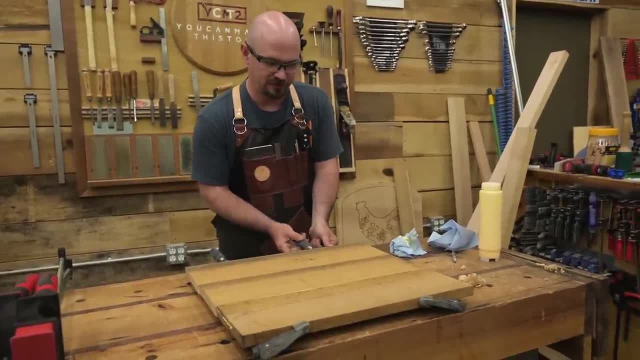 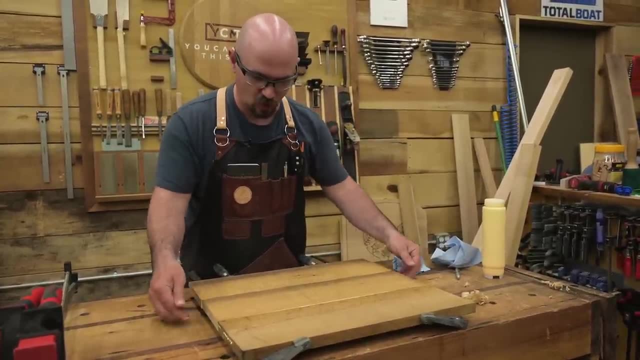 oh, but you know I've been reading and I know those are expensive. but one of the things that makes parallel bar clamps so awesome and rather expensive is how much clamping force you can get. You can really get a whole lot of force on there. 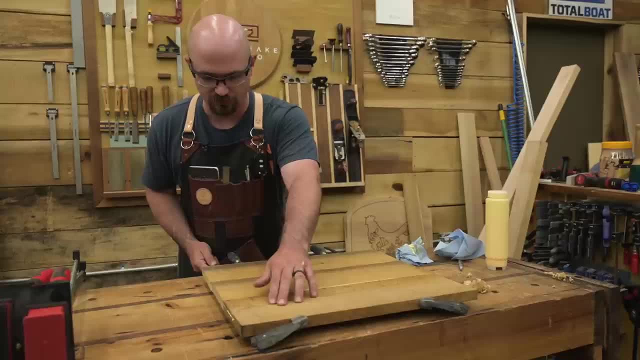 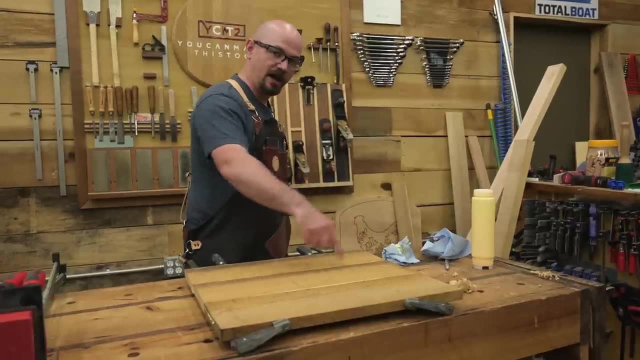 and doesn't glue need just an absolute ton of force? No, it really doesn't. You only need a ton of force on your glue ups if your boards are milled improperly. If these aren't nice and straight and you're trying to force the 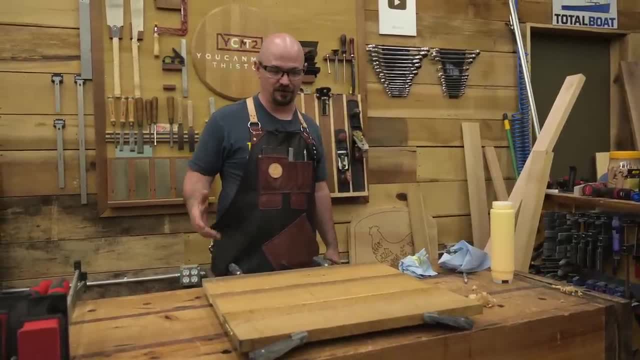 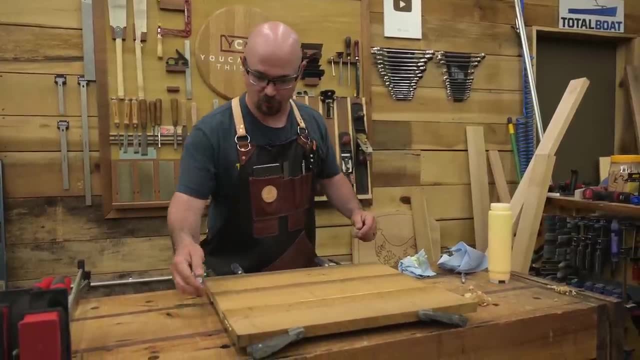 boards together because they're not straight. that's when you need tons of clamping force and that makes a much weaker glue up. Just a little pass hand tight is all glue needs. to set up well and give you a good glue bond With these. 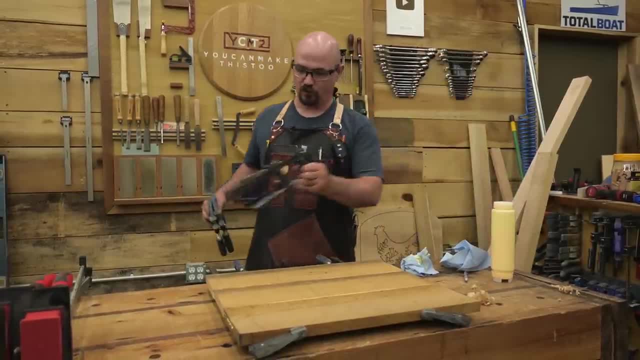 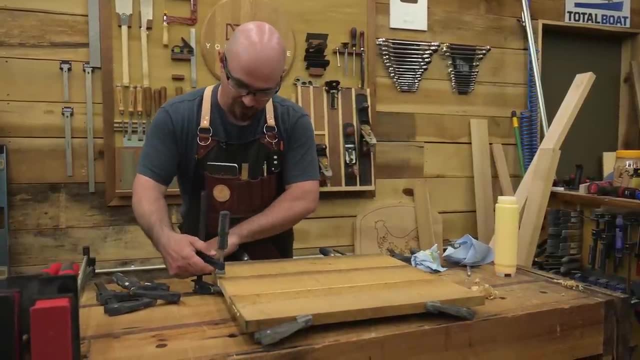 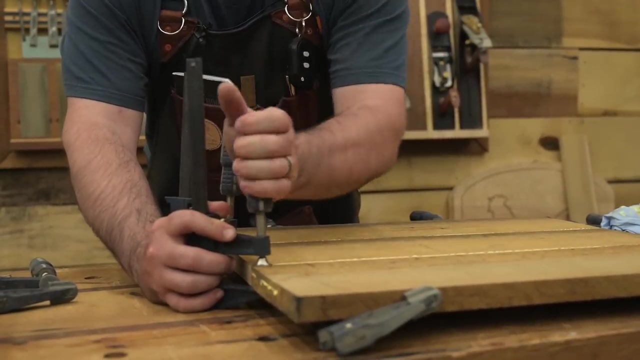 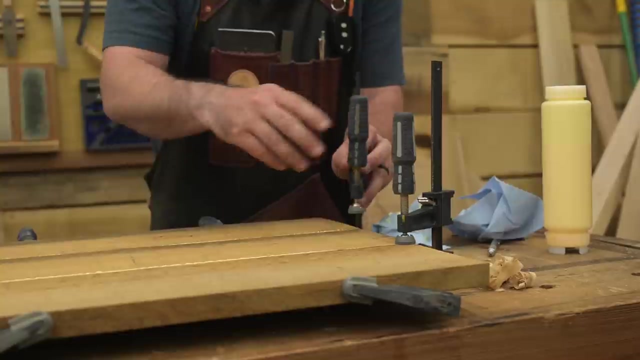 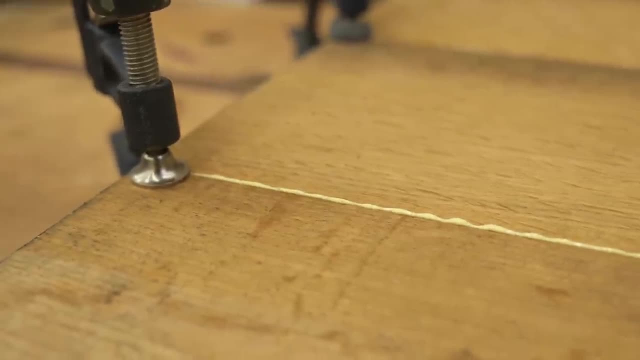 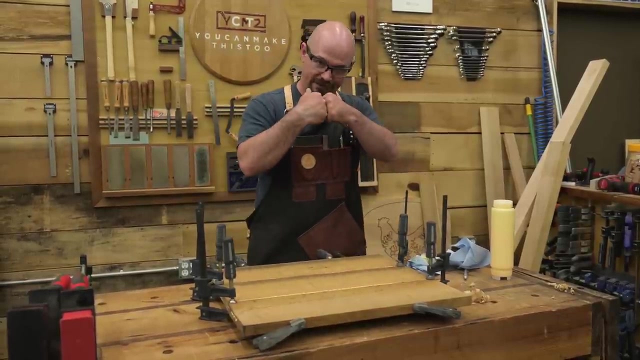 ups is your squeeze out. honestly, this much squeeze out just means I used more glue than I needed to. but the other thing it does tell us is: this is nice and flat. if we have even squeeze out, that means we have equal pressure across the across the whole joint. but you really definitely don't. 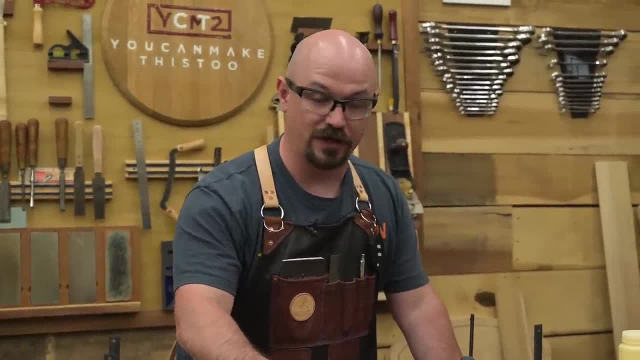 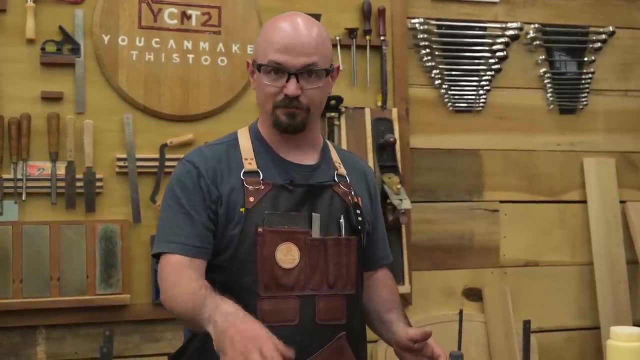 want to see. it's like a lot of squeeze out in some areas and then no squeeze out or even gaps between them. that means your boards aren't touching and PVA glue- most wood glues really, especially PVA polyvinyl acetate- is not a gap filling glue. what it does is help bond surfaces. 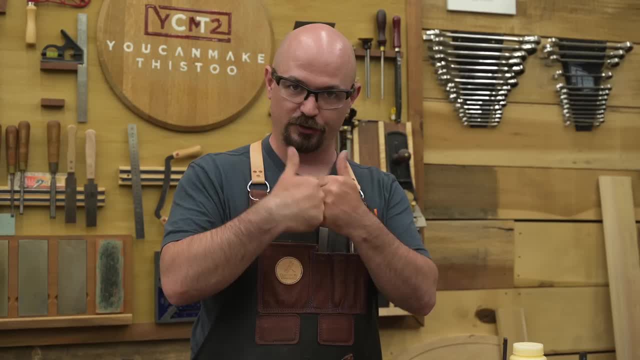 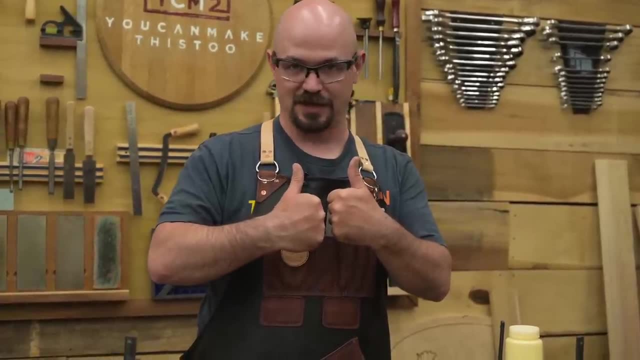 together. so as long as they're physically in contact with only a little bit of glue, kind of be in the medium, it's going to have a fantastic bond. but if there's a gap and it's trying to span that gap, PVA does not do that. it's not going to be strong. but so long as they're. 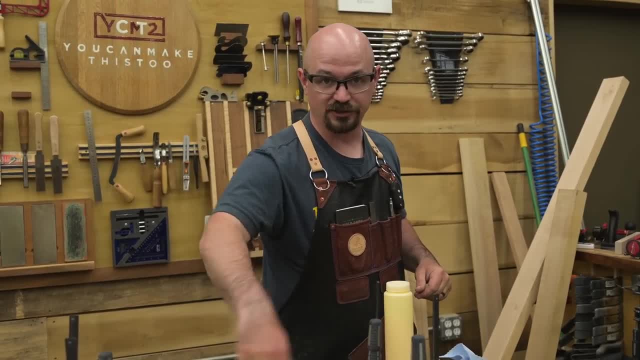 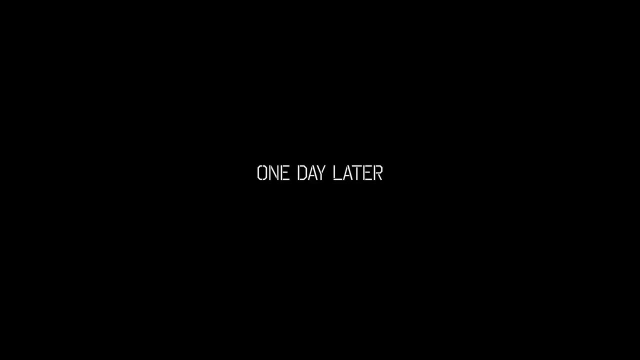 touching, you don't need anything else. on a long grain edge to edge glue up like this wood glue is plenty strong for any purpose. I actually clamped this up at the end of the day, the yesterday, so it's had overnight to sit, which I try to do with with my glue ups. 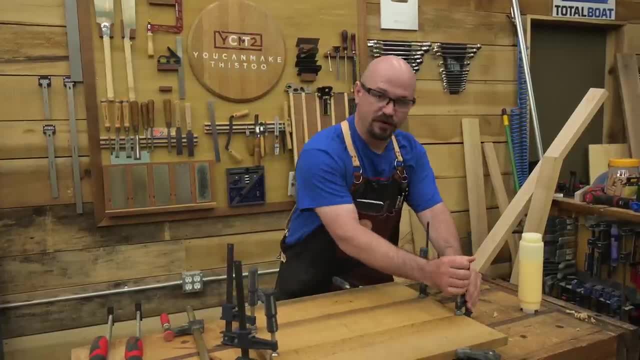 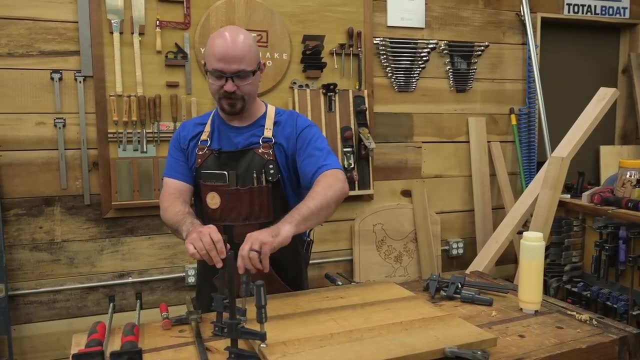 and if you don't have a lot of room in your shop, that's always a good tip, because then you don't have to worry about trying to. you know your glue up being in the way, especially if you do it on your work surface or something. if that doesn't work for you, though, then realize most PVAs only. 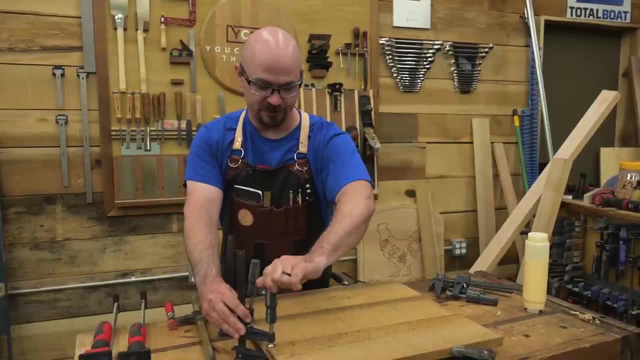 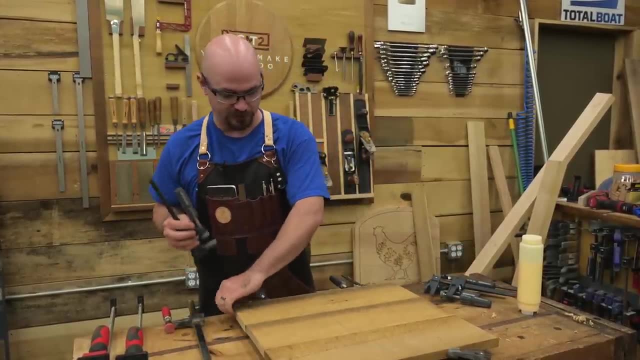 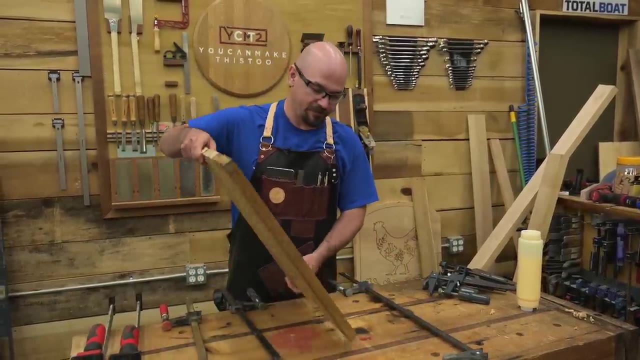 require about two hours of clamp time and then you can unclamp it and especially on three-quarter inch material like like this, I've definitely many times when I've been in a hurry only done the two hours: pull it out of clamps. glue does take upwards of 24 hours to fully set for regular working two. 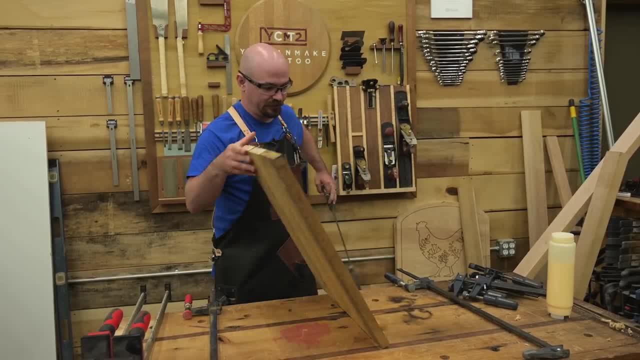 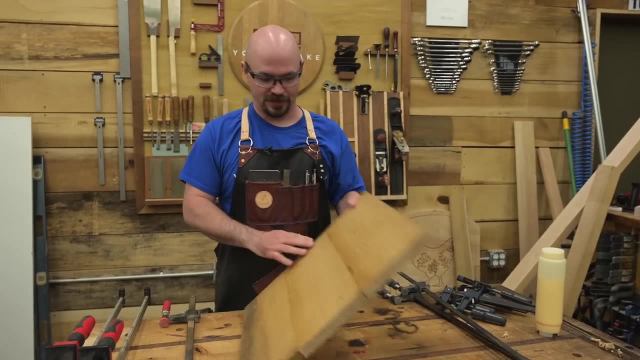 hours and I've been able to run it through my planer, through my sander, start cutting it down and reshaping or whatever. what you don't want to do is, after two hours, take it off and then start like beating it against stuff. we've got a panel. now let's do some scrapage and then get some. 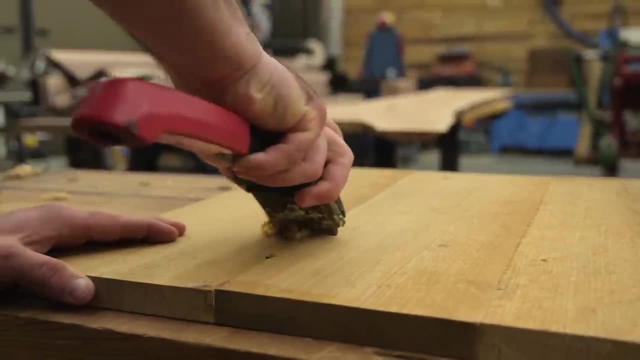 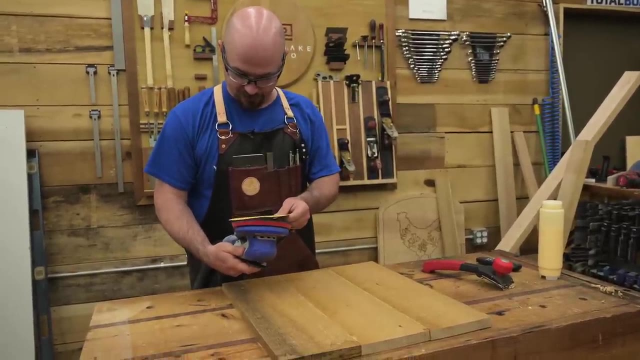 initial sanding done on this. this is pretty rough, so I'm going to start with 80 grit paper on my sander. that's pretty aggressive and will help smooth things out pretty quick now if your glue up isn't perfect, got any issues and this will fit pretty well. I'm going to start with 80 grit paper on my sander. that's pretty aggressive and will help smooth things out pretty quick now if your glue up isn't perfect, got any issues and 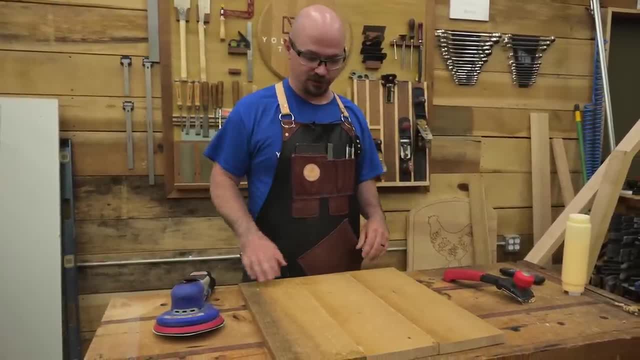 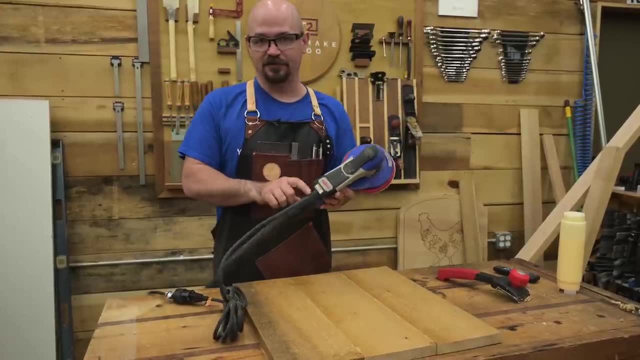 through your planer and you have a planer, you can by all means do that to smooth things out, but you can also do it all with the sander, obviously. I'm blessed to have a really nice sander from surf prep. whatever sander you have, if it has any kind of dust pour and it might have a bag, take the bag. 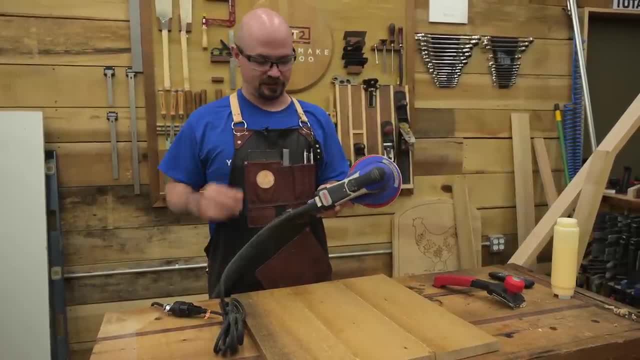 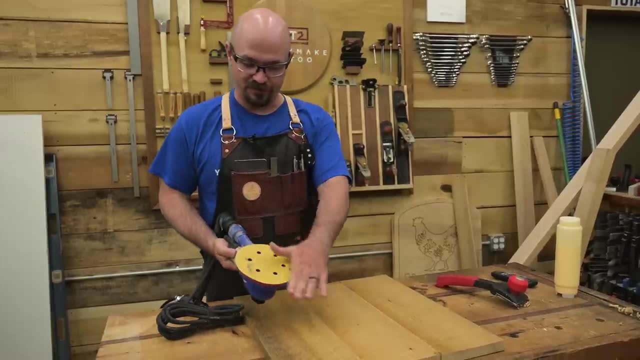 off and sometimes there is a vacuum attachment in there. even if you don't have a dust collector, just hooking a sander up to even a shop vac goes a long way in improving your sanding performance. because what happens if you're not moving the dust out from under your sanding pad? here is 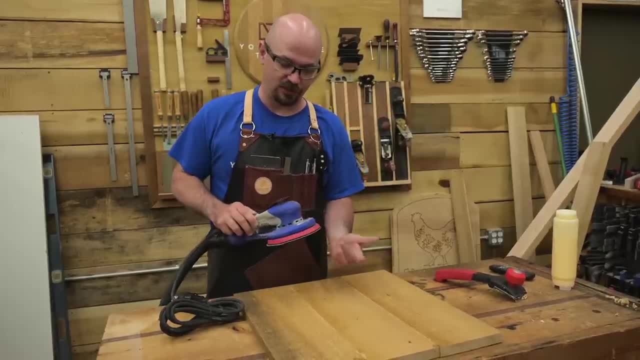 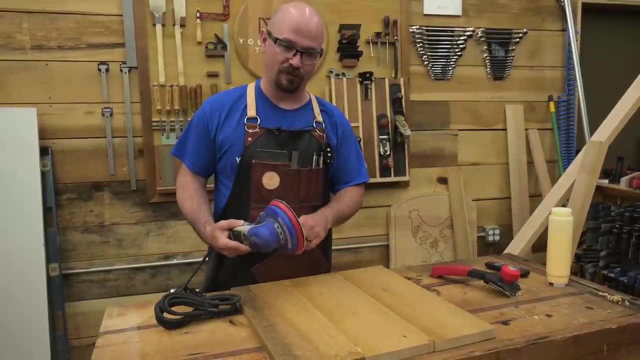 you collect a pile of dust which builds up heat, and then you're. energy and work goes into just putting heat into that pile of dust instead of moving it away. and heat is the enemy of sharp. so you dull out and wear your paper a lot faster and you're. 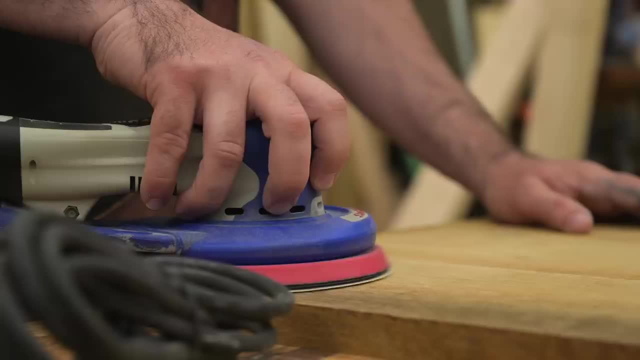 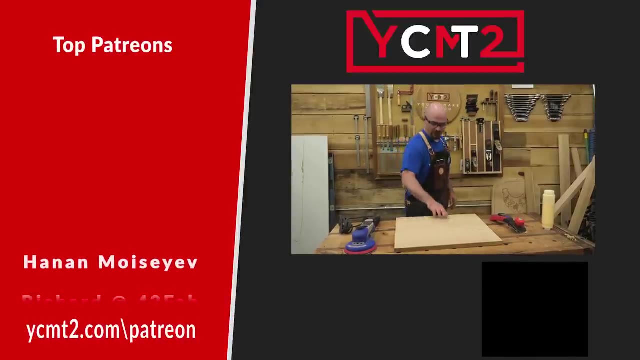 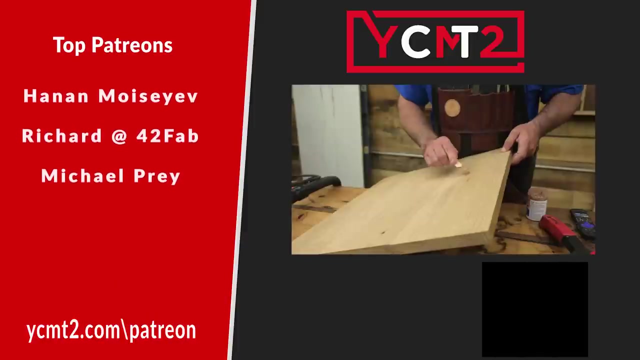 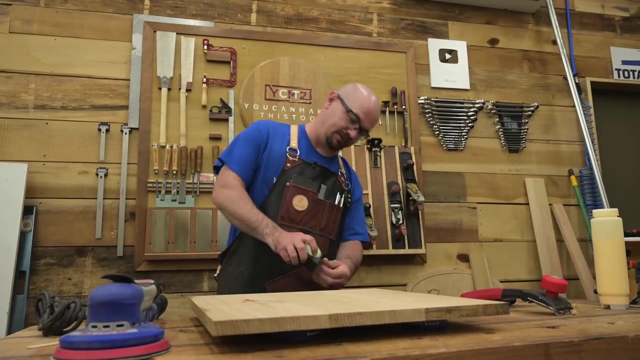 not cutting as well, because you're just regrinding dust instead of cutting your surface. all right, now I can see my wood got a good feel for it. I see anywhere I need to fill. let's get some filler on it while the putty dries. I'm going to go ahead and get started on the legs now. I thickness here three. 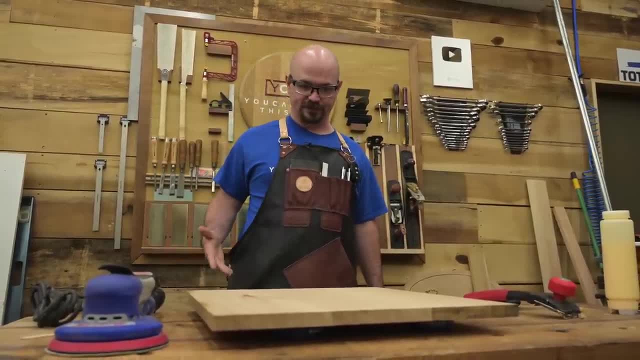 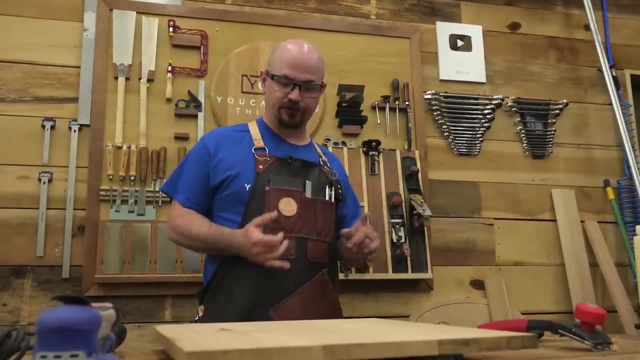 quarters of an inch. perfect. I know I want the top of my table will be 26 inches for this little side table, so that means 25 and a quarter is the length I need my legs to be. if you're doing like a dining table or anything like that, 30 inches is pretty typical, like 30 to 32 normally. 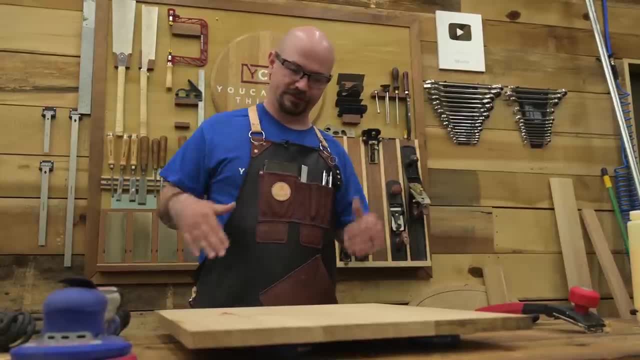 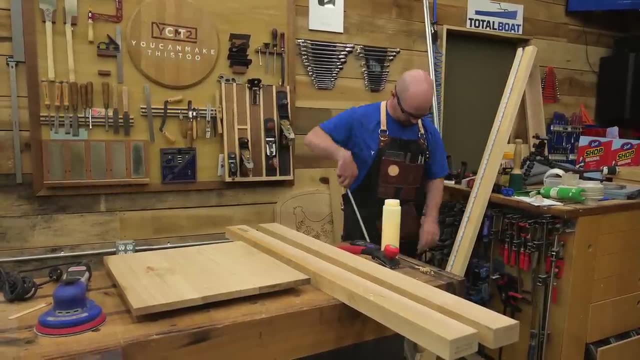 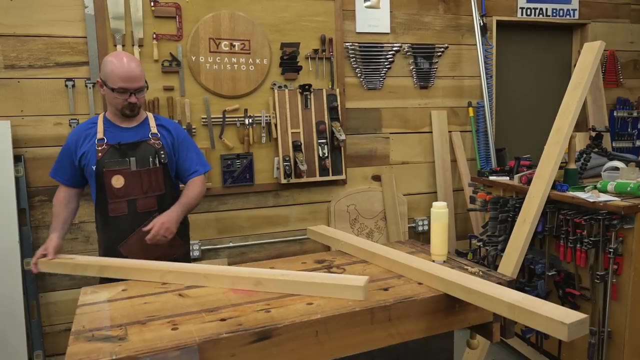 30 side tables, anywhere from like 18 to 26, just depends. just go measure where, where you want it to. I'm just using scraps, as I mentioned, so none of these are the right dimensions I need. so just use the circular saw, table saw to break them down to leg shapes. and again, if you don't have the tools, 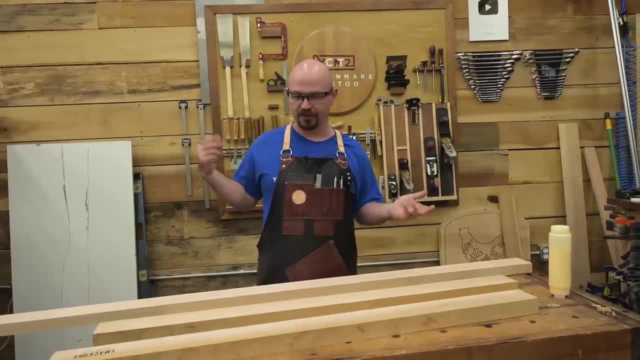 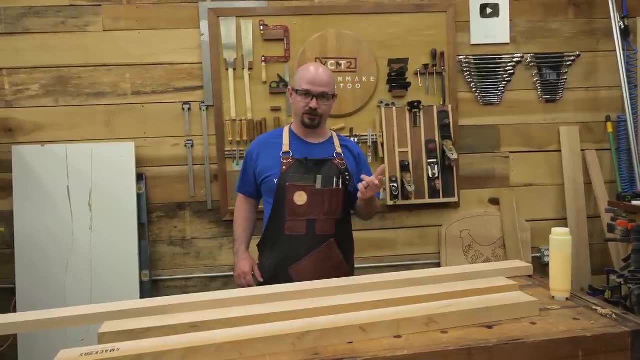 to do that, just buy wood about the size you need. so for a table like this, some two by two be great size for legs. or since you can do a glue up and those clamps are great for it, you can always get two one by twos and glue them together to make a two by two or something. lots of ways to tackle. 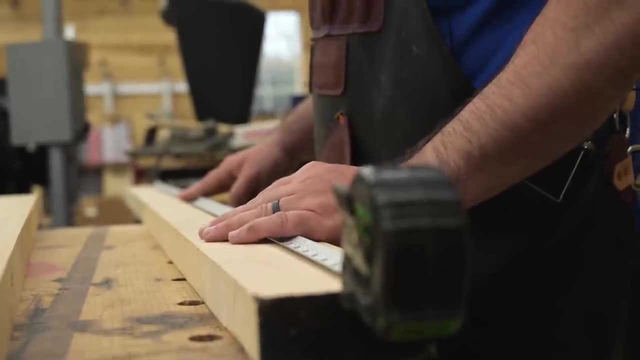 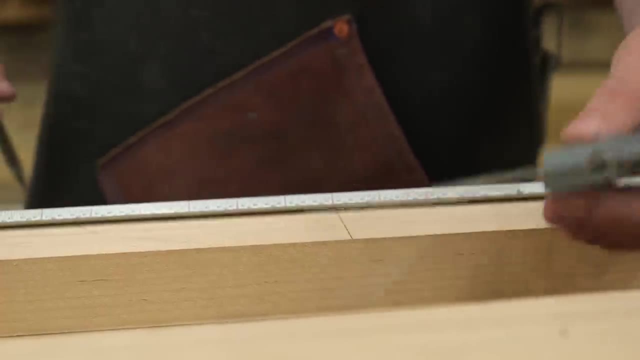 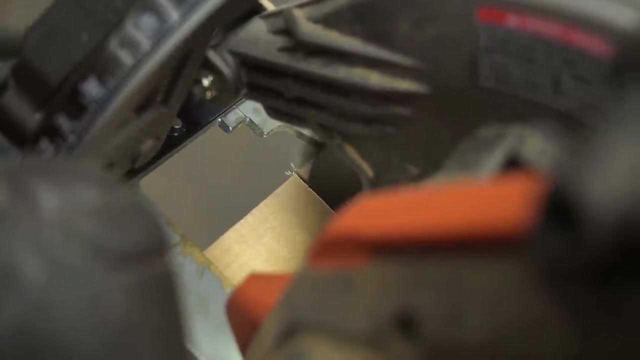 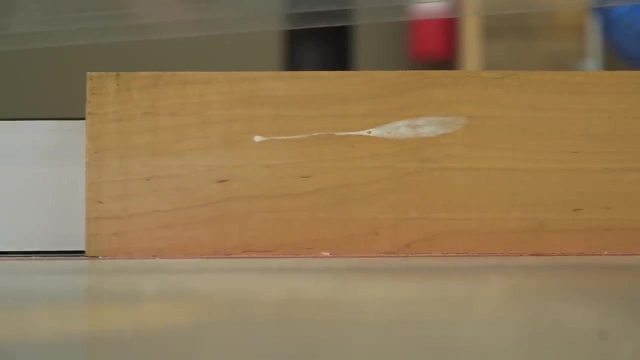 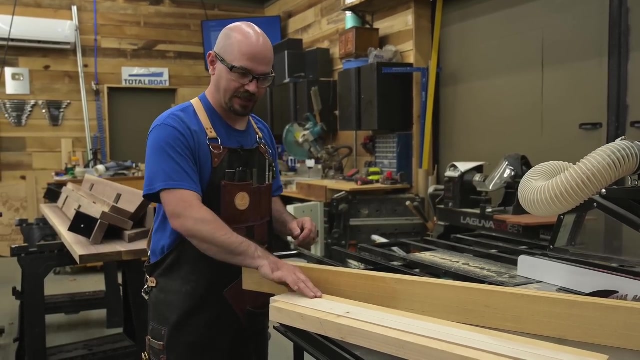 it. god, I'm an idiot. there's plenty with this, because I can do side by side over. I would. I was geez, so I took the stock I had. now I have four squares. I only need three legs. another great trick: if you have the material for a table, I don't know how many I need, three is true. 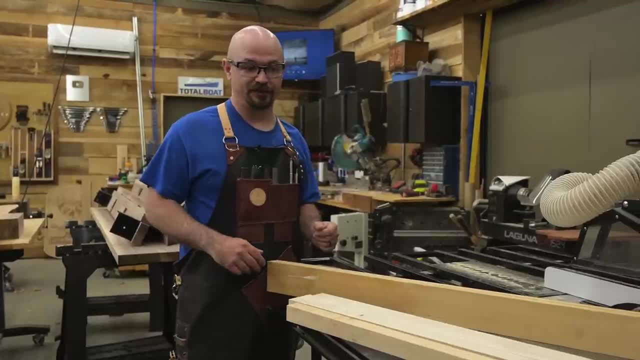 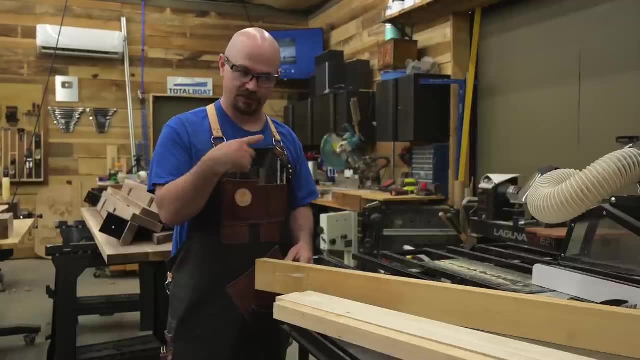 make duplicates of parts you can sub in in case you mess up one leg. you've got an extra leg blank, or you know I have way more material here for the aprons which is gonna go between the legs and under the top. then I need so that way. if 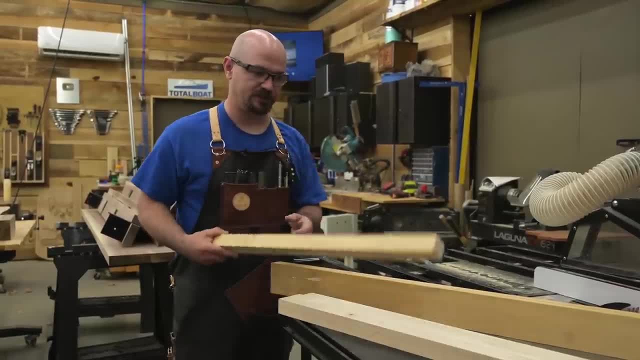 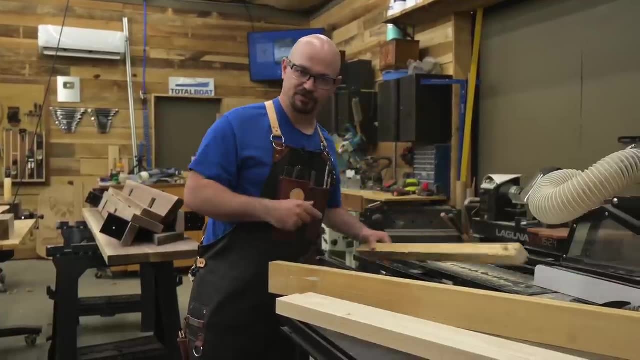 I mess up a piece I have extra ready to go. two tricks I can use at the table saw here was to make my squares instead of relying on any measurements. you notice, I stood it up on edge and set my fence to the thickness of the board. so then when? 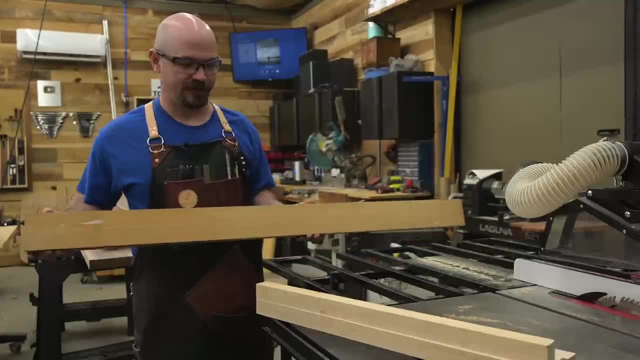 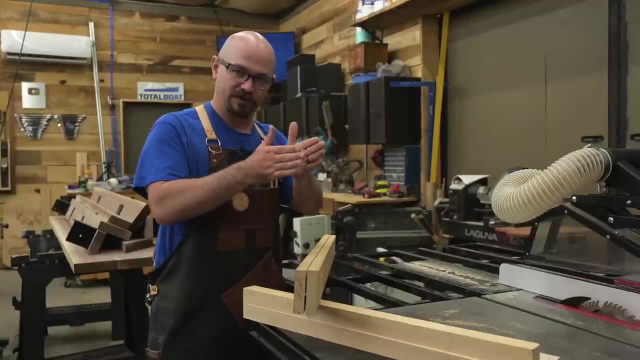 I laid it over and cut it. I have a square also. you notice I use the table saw to resaw this, make it thinner, and I could have cut all the way through, but I left a little paper here. it helps make sure the board doesn't like bind on the. 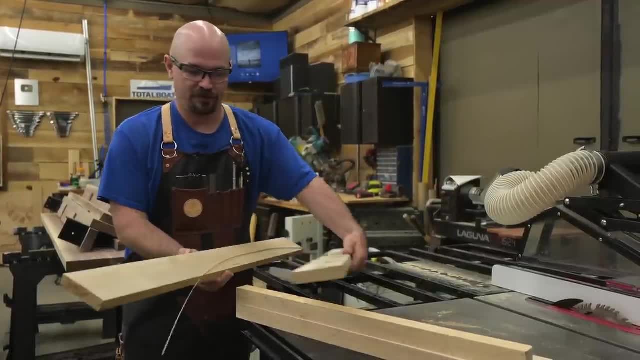 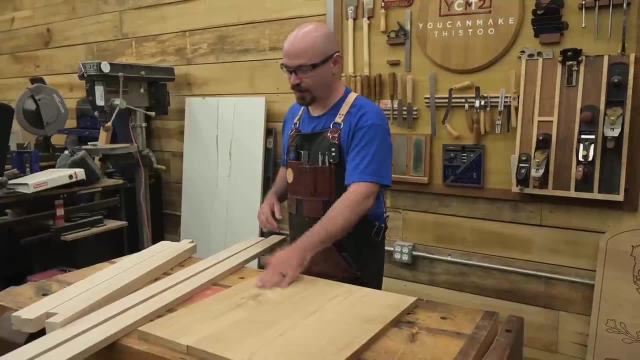 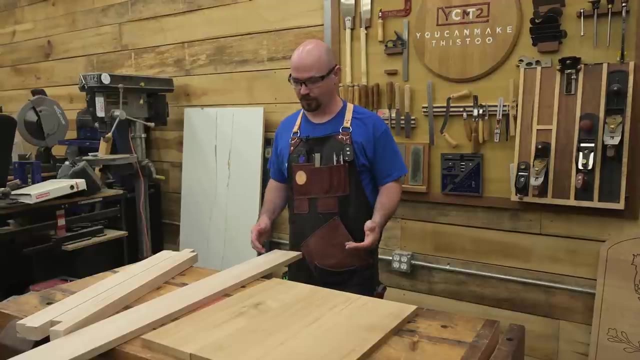 blade or flop around, create a hazard, but with that thin little paper it just snaps right off, but it holds it together. quick pass with the sander and that little Ridge will go away. putty dried, everything is sanded now to 150, so pretty much finished, ready now. we just need to bring it all together now. if you. 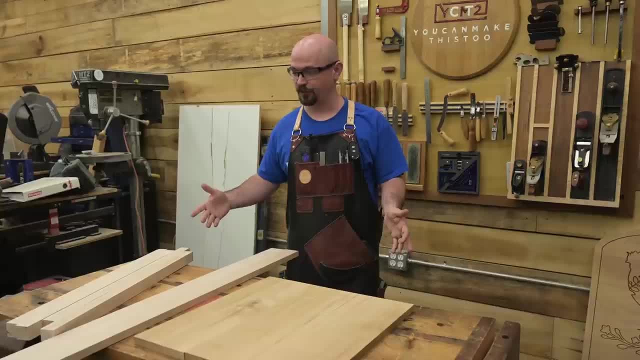 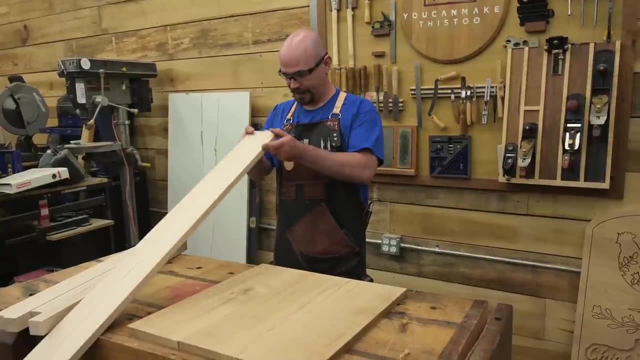 didn't have saws and you wanted to take the super easy route. this is basically where you'd you'd start: go to the store, buy wood, the right dimensions, and now you're ready to start bringing things down to final size. I did rip these down. I want to say they. 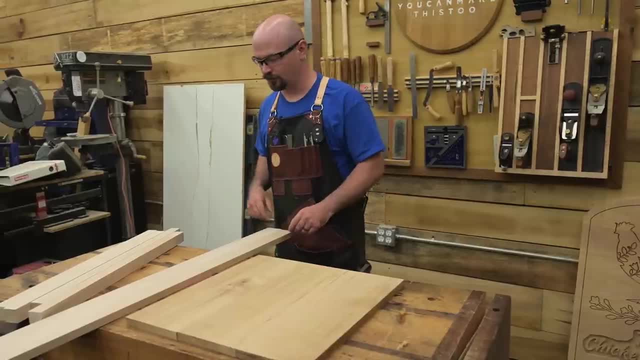 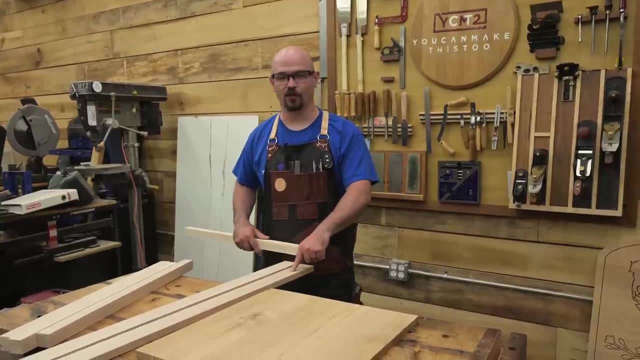 were originally three and a half. then I went to two and a half. that still didn't quite look right, did a little math and ended up cutting them down to two and a quarter, because these are about one and three eighths, with one and three quarters to two and a quarter. that is very, very close to the golden ratio: 1.62. 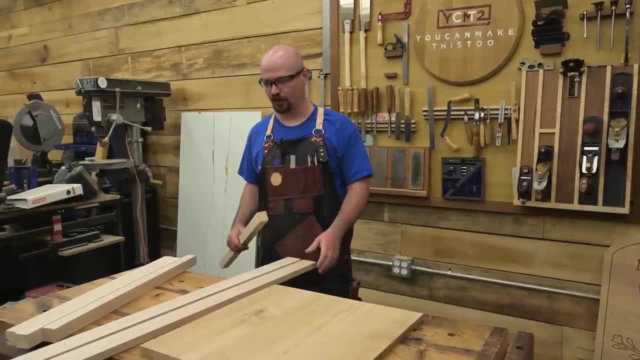 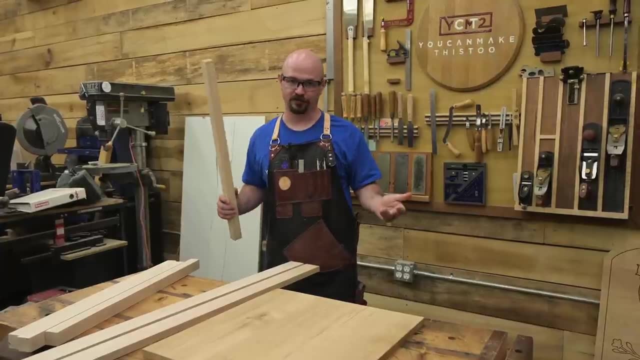 so if you're ever like I don't know what size things are gonna look right, or if things don't look right, use a golden ratio. so all they just took this is a square, so it is one and three eighths inch wide, so took one and three eighths. 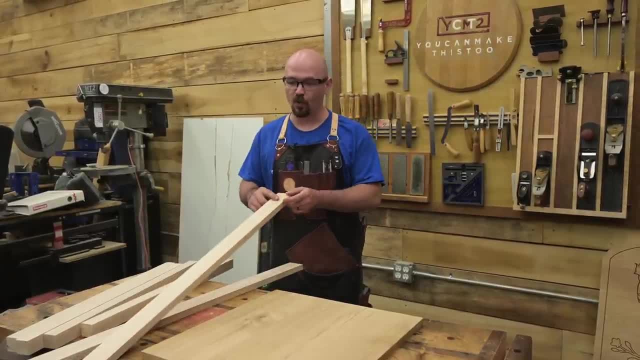 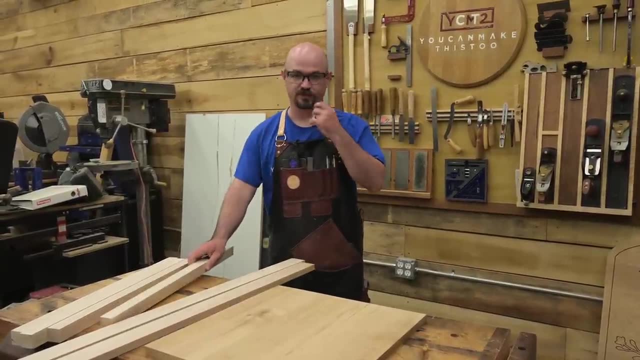 multiplied that by 1.62, it gave me just under two and a quarter. I just rounded up to two and a quarter for ease, and now when I hold these beside each other, I'm like that looks balanced, that looks right. so that's, I use a golden ratio to 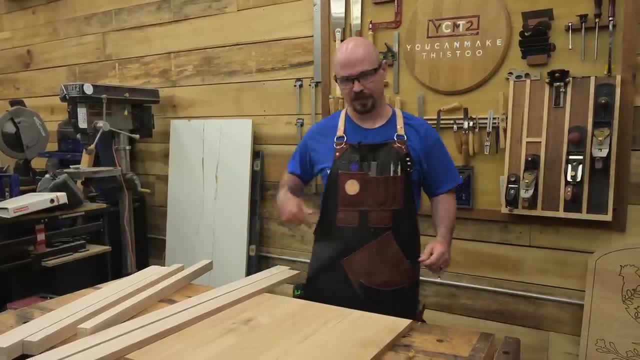 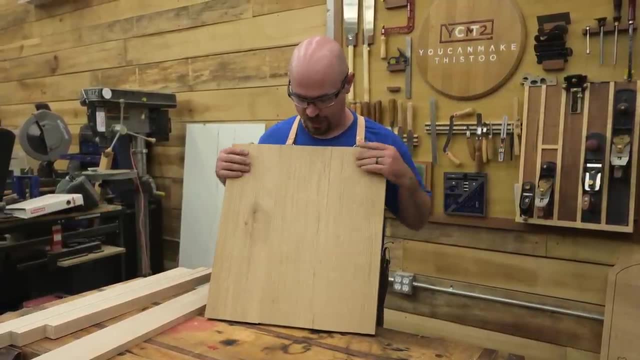 solve any dimensional problems a lot of time when it comes to aesthetics, so keep that one in your pocket. as I mentioned, we're doing a triangular table and obviously this is in the triangle. so the next step is going to be marking out our triangles, and I think I want to try to work a lower shelf into this. so 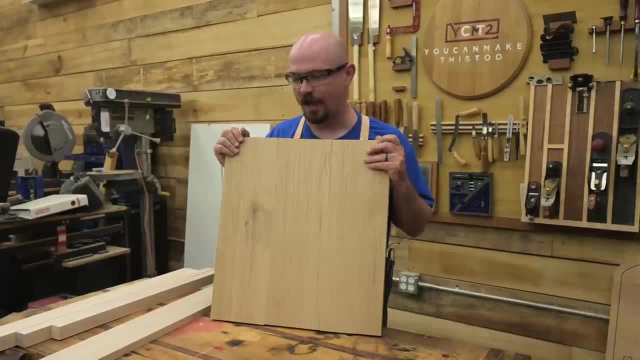 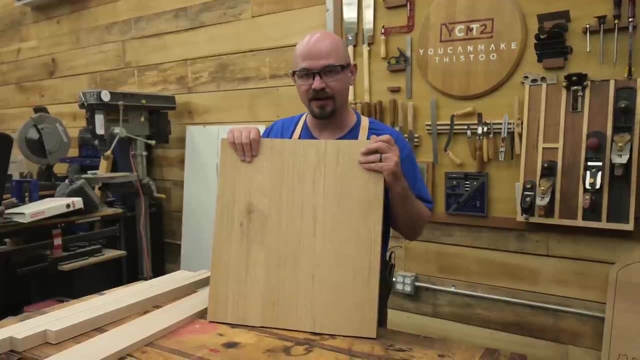 mark out the triangles for the top and the bottom shelf. how am I going to join the bottom shelf? there's my secret. I don't know yet. don't worry about having everything solved when you build sometimes. just get in there and if you have 90% of it figured out, you'll figure out the last 10 when you get to it. so 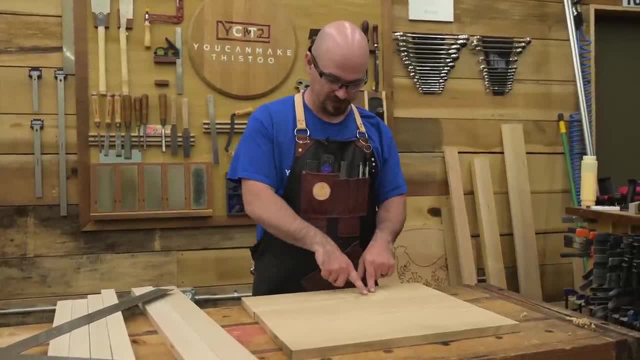 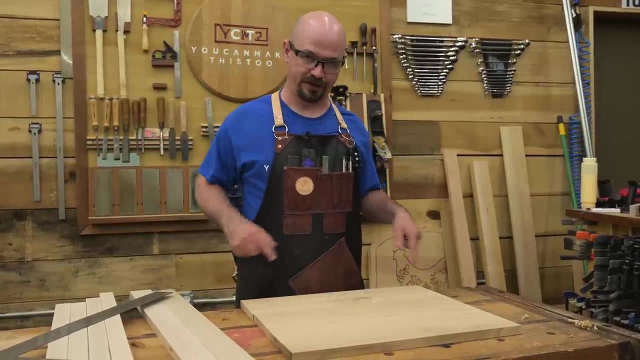 I'm just deciding what part of this I want to be my top and front, and I kind of like this little defect here, so we're gonna leave that. it's figure, not a defect. now, in my experience, true, triangular tables are just really too harsh with all those sharp corners, so we're gonna. 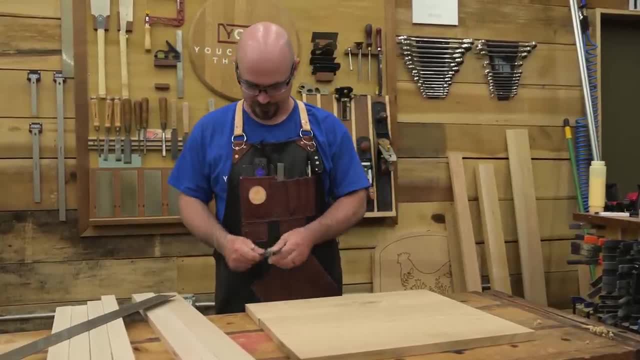 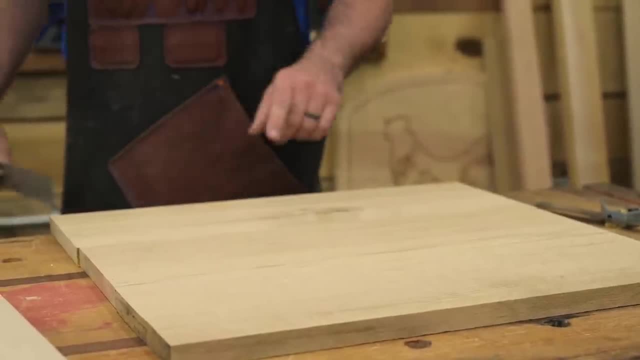 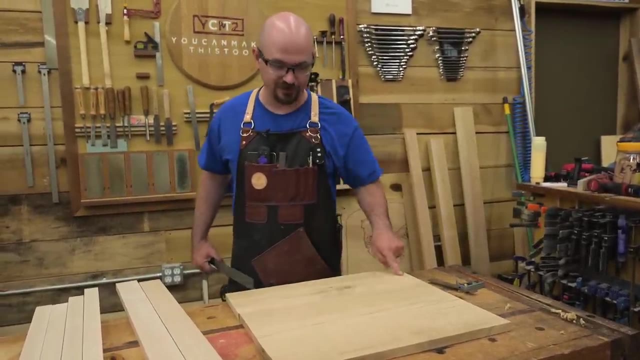 ease that up a bit by giving us, let's say, a little inch on the ends. that will come in, okay. so now I have a 1 inch mark and I actually don't know what this dimension needs to be for the front edge. what I do know is my two back legs are 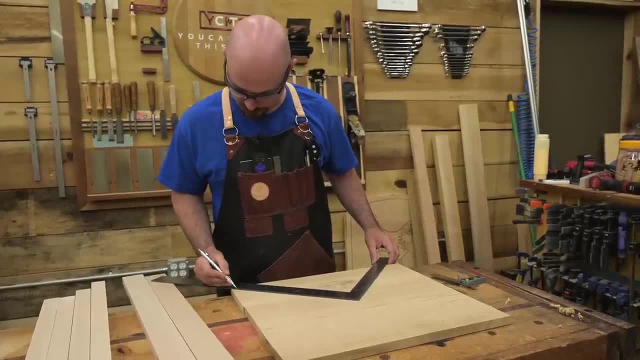 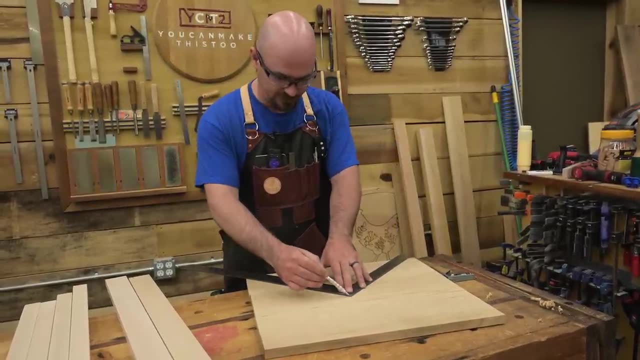 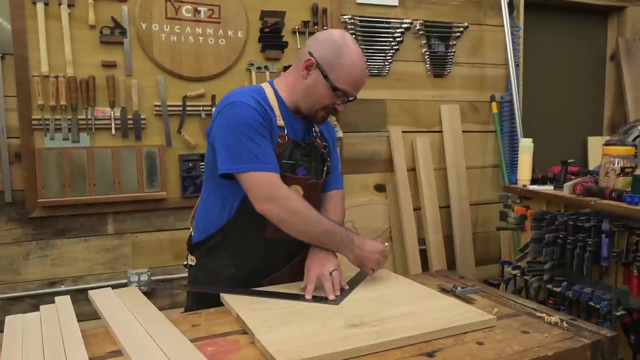 13 inches, but just using my big old framing square here, I can just put 13 and put this there. I was actually really close to where I need to be, so, yeah, I just put both the 13s on here. perfect now for my bottom shelf. I'm not gonna add that little bump out because I 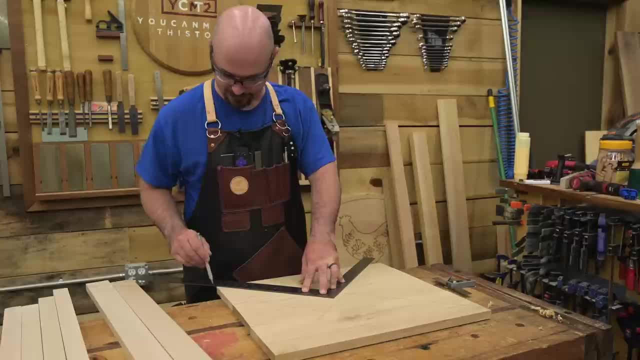 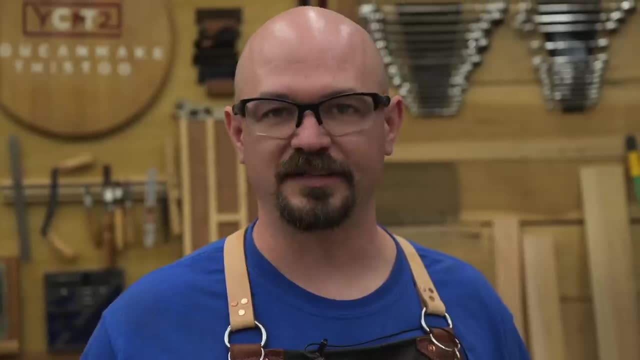 have a feeling it needs to be a little smaller anyways to fit inside the legs. so I'm just gonna do 13 and 13 right off the front edge, you know. I've got two triangles ready to go now. I've already said it: take the principles, not the. 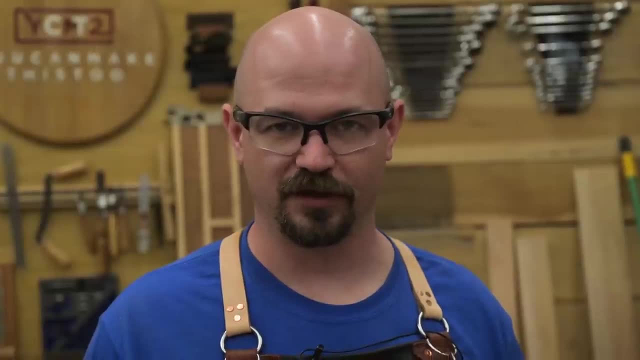 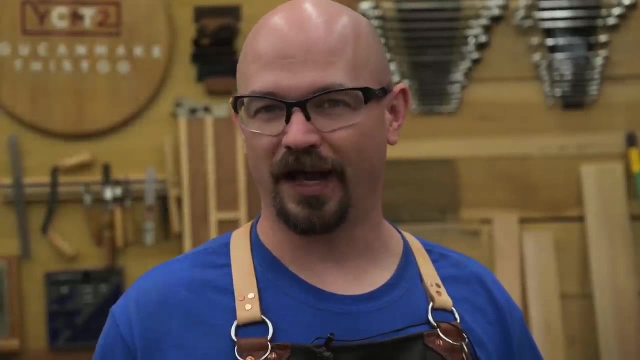 design here. you can take these principles and make any table with any number of legs, any size, etc. I'll give you a hint, though: if this is your first table: a three-legged table always sits perfectly in front of the front edge. four-legged tables can rock. so then there's some tricks. 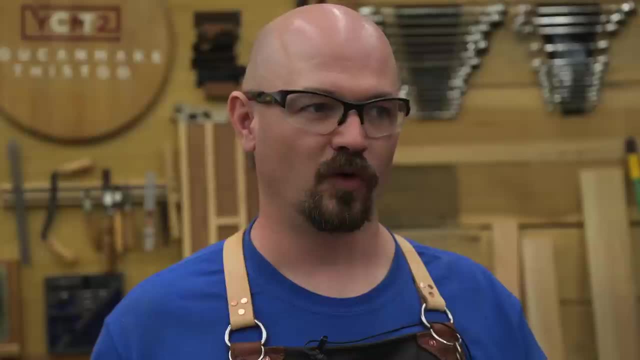 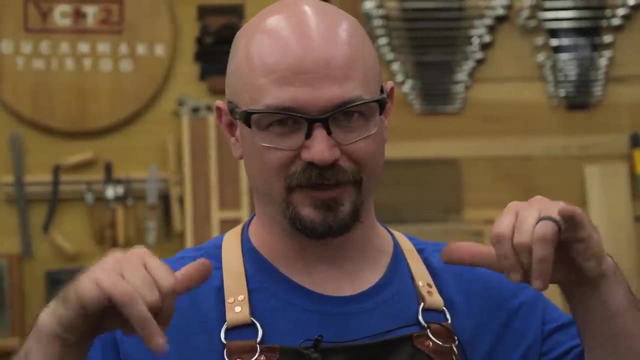 on making sure that they sit flat and use adjustable feet, or play some tricks on the table saw or just sand them. The problem is not all floors are flat. so even if all your legs are the same, if the floor isn't flat, you're not gonna run into issues. 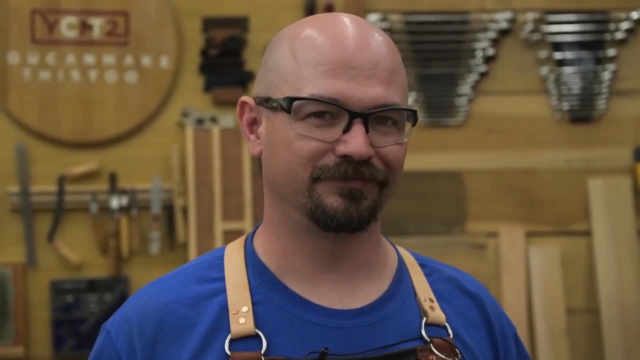 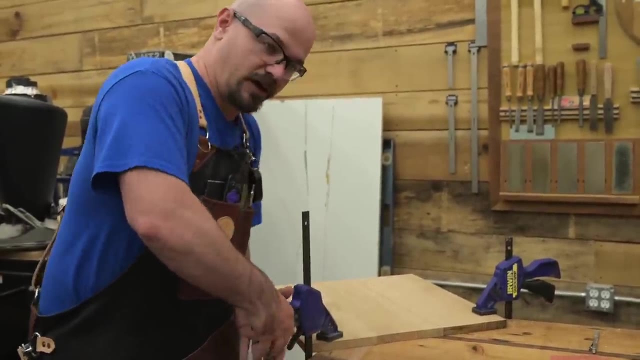 so adjustable feet is good, but three-legged tables always sit flat, Since these aren't rough cuts, these are my finished cuts, two dimension, and I'm not gonna be making any more cuts. I wanna be really good. This is where a friend that can hold things is really handy. 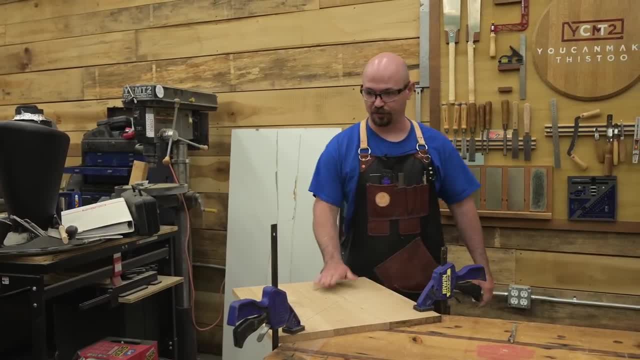 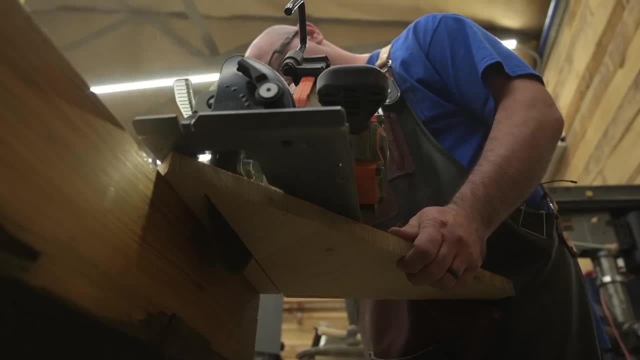 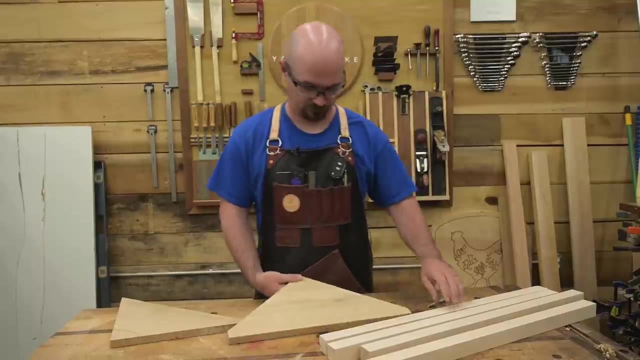 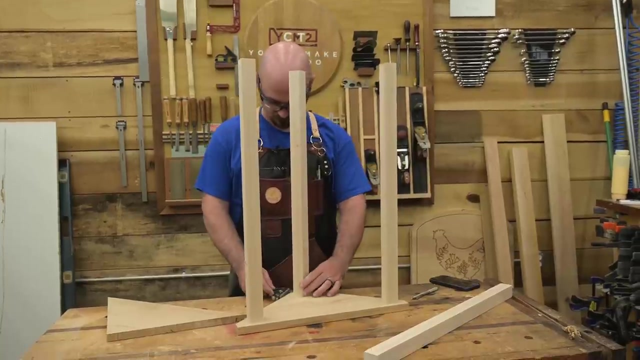 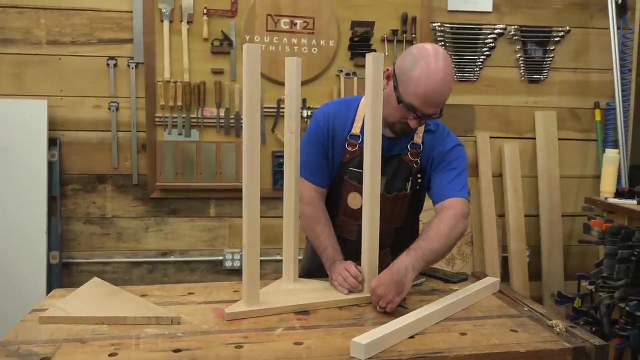 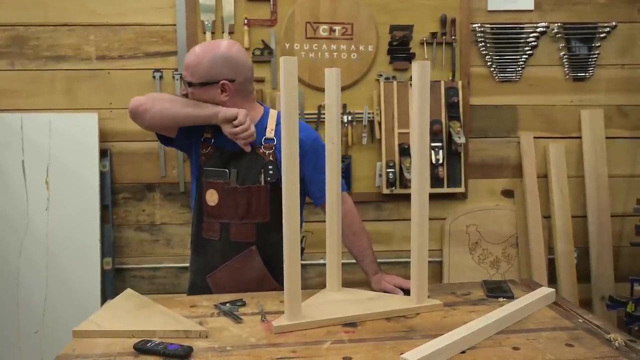 but if you're working alone, just break out whatever clamps and find a way to hold your piece. Look at that. we got two triangles, So figure out my locations on all the legs. To figure out the locations of all the legs: 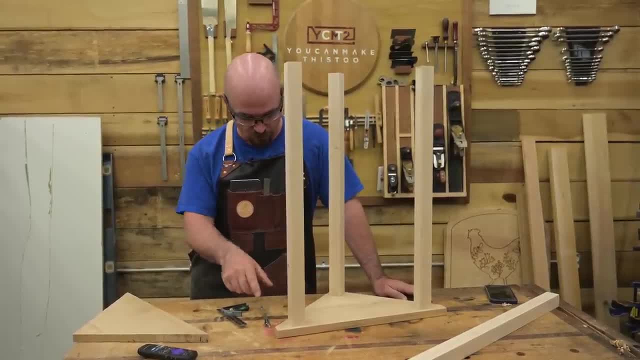 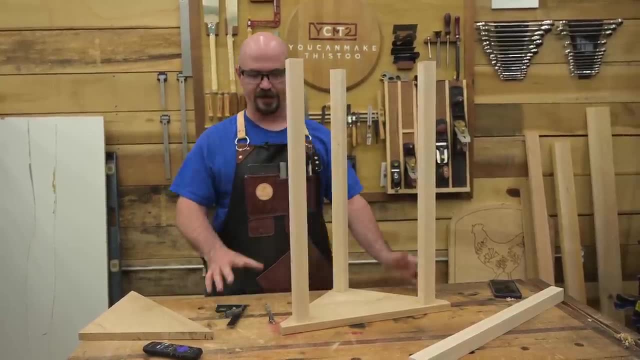 I just flipped the piece upside down because this is where the legs are going to go. Wanna make sure the reveal is all the same. I started with a three-quarter inch reveal, which is pretty common, but I normally do larger things, and it just didn't look right. 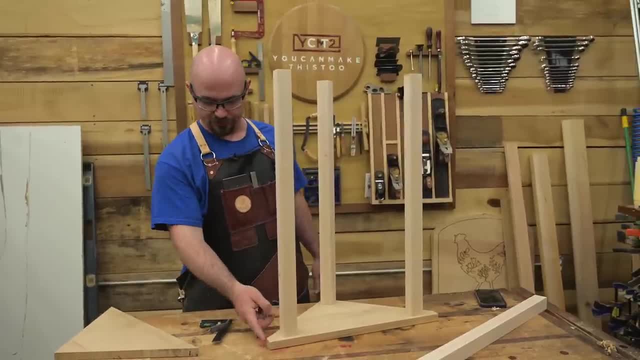 and everything was way too close. Oh, it needed to be smaller. duh golden ratio. The thickness of my table was three-quarters of an inch, so I did three-quarters of an inch instead of multiplied by one-sixth two. 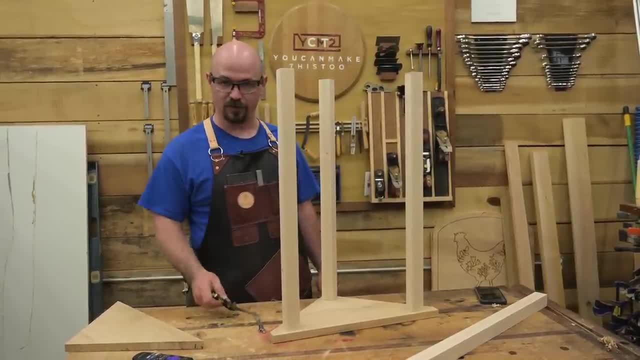 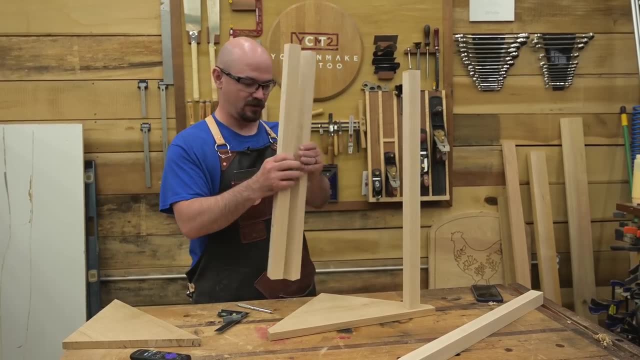 I did. divided by one-sixth two, That was just under half an inch. so, bump, my combination squared a little under half an inch, set everything to just under half inch reveal and this looks really good, And now I can move these out of the way. 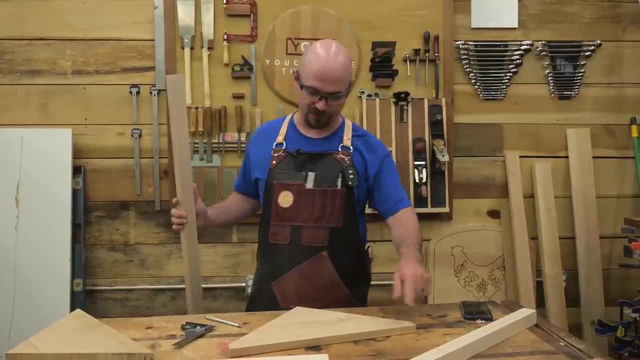 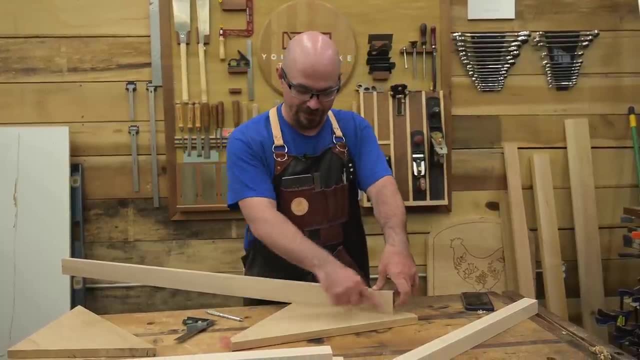 One of the tricks in woodworking is to measure as little as possible. So, having laid everything out this way, I can actually take my board and make my marks directly in place and never worry about what any of these numbers are, because I bet they're really weird fractions. 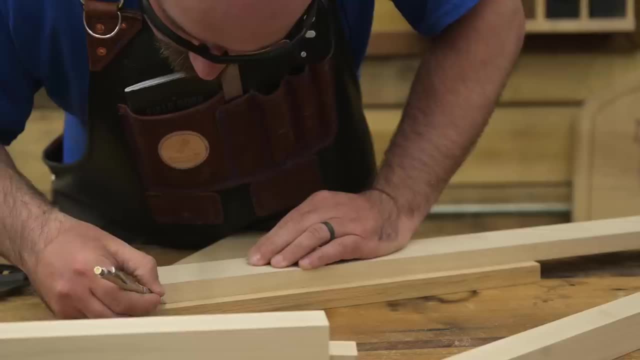 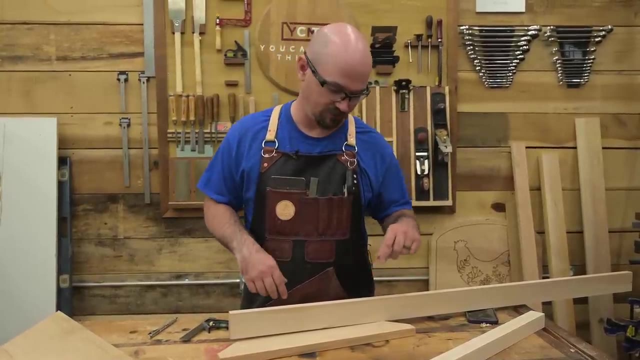 But if I just mark exactly in place, it's gonna be right. Another thing that really helps how your projects come together is remembering the relationship between the line and your cut, Because these lines, because my pencil lead has thickness, are marked on the outside. 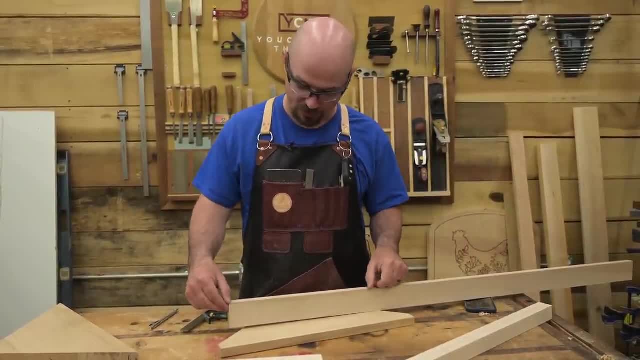 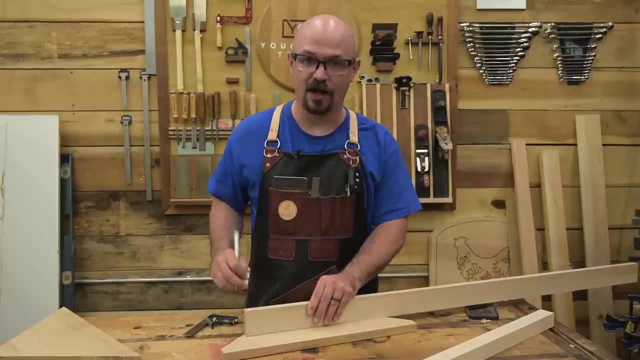 and I transferred that exactly. when I cut this, I actually want to make sure that pencil line is still there. I don't wanna cut it away. The way I help myself remember that is I put an X on the outside of that line. 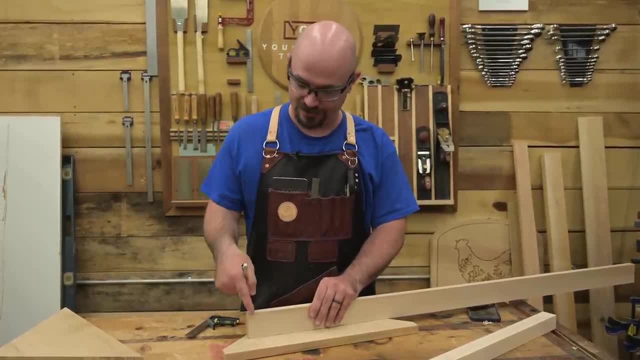 and now I know that line needs to stay. If I put an X on the line, that means I need to cut exactly on the line and the line goes away. If I wanna be on the other side, I put an X on the other side. 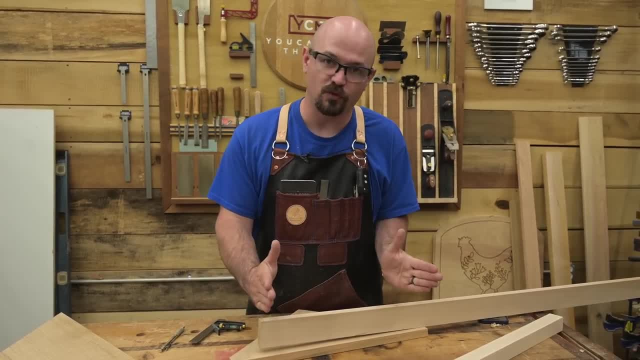 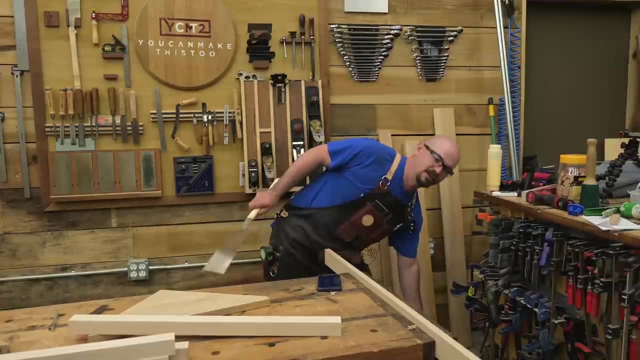 Because if I cut that pencil line away, this would actually be a little shorter than when I need it to and it'd pull in my legs a little bit. This is a construction tool and I know if I use that to make these fine final cuts. 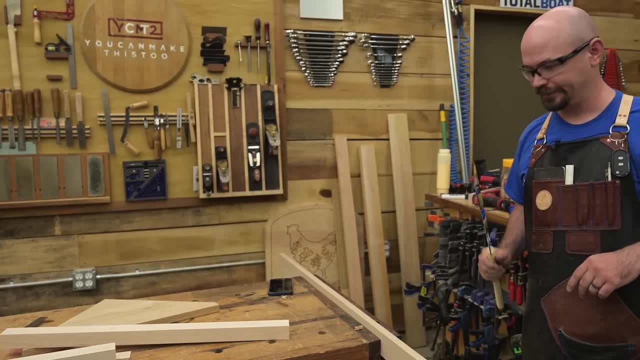 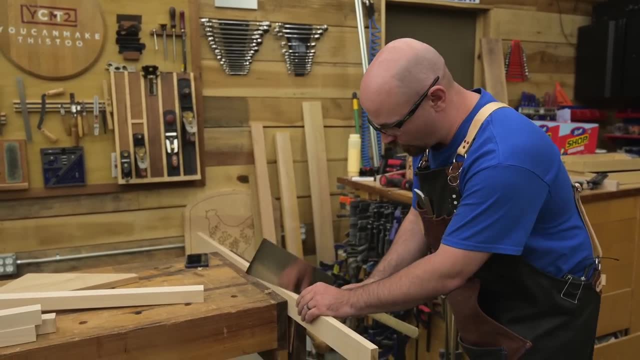 I'm not gonna be happy with how clean it comes together. Sawing straight by hand is not hard. The biggest thing is you wanna just make sure your body's out of the way. here it's easier to move straight And the trick to being square. 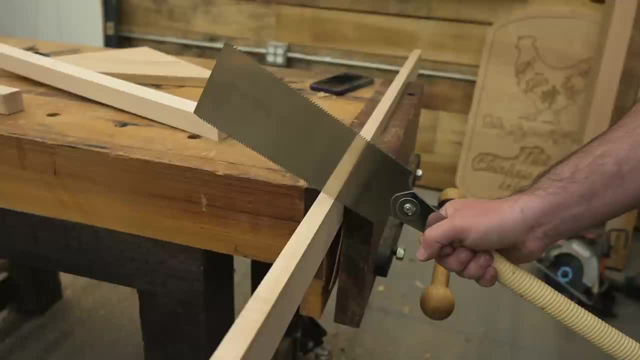 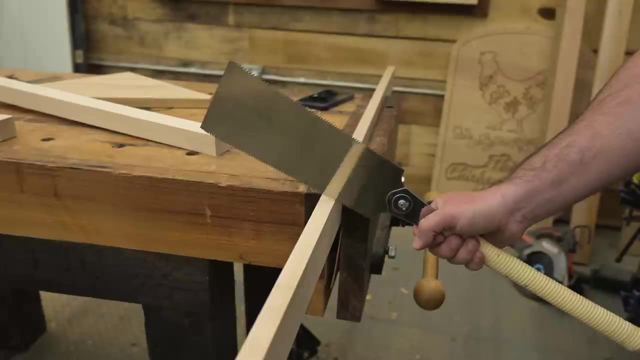 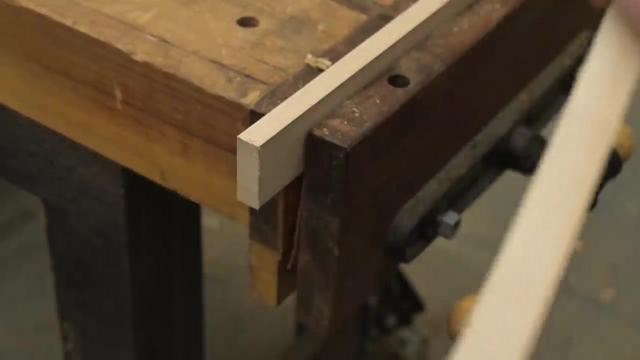 is actually to use the reflection in the blade If the reflection of this corner lines up perfectly with the corner on the other side. I'm straight. As I move away from straight, I can see that in the reflection. The other thing that helps not be intimidated by sawing. 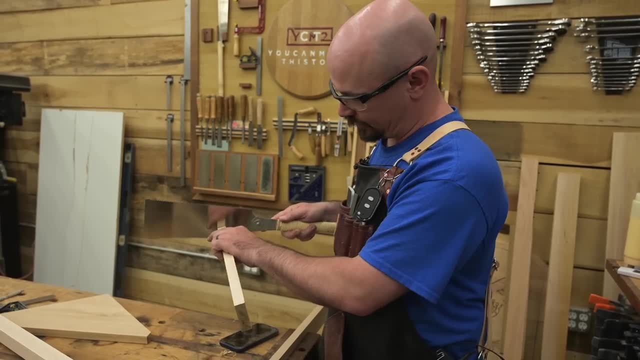 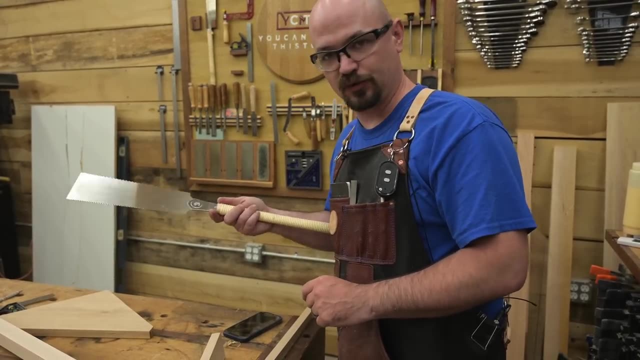 is realizing. you really only need to be super concerned about the first inch. As we get deeper, you notice I have a wide blade. so once enough of this blade is in the cut, it's gonna keep itself going straight cause it can't really twist much. it'll bind up. 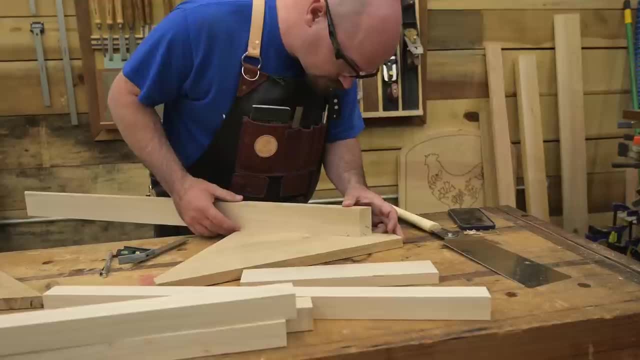 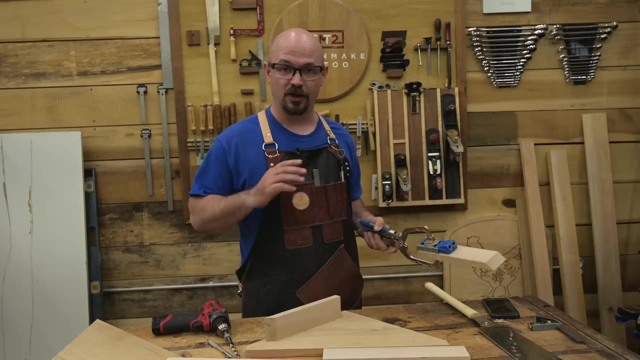 All you gotta do is really worry about that first inch or so, and the rest will take care of itself. Now, as far as bringing this all together, we're gonna use the infamous Kreg pocket hole jig- The only thing I'm gonna make sure I do. 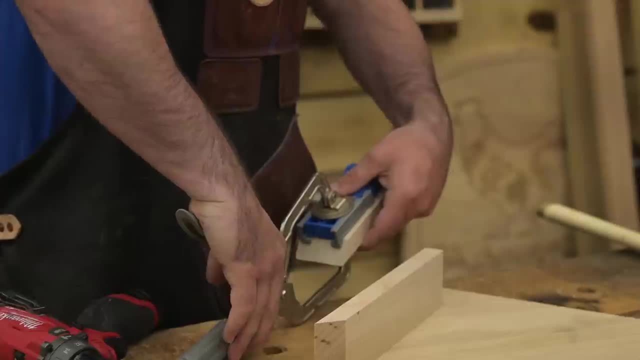 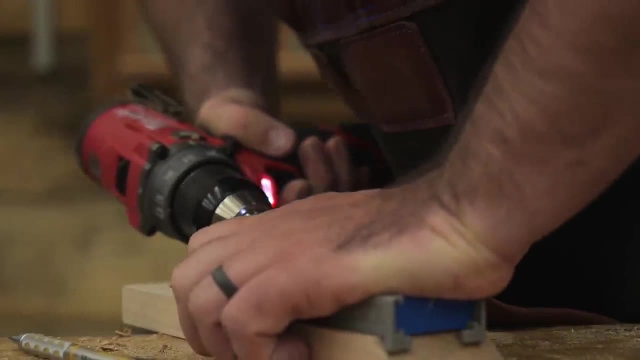 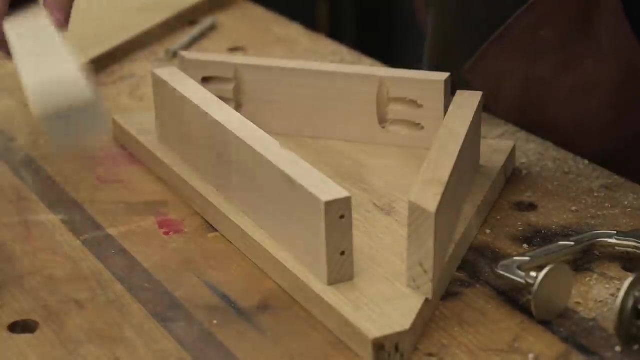 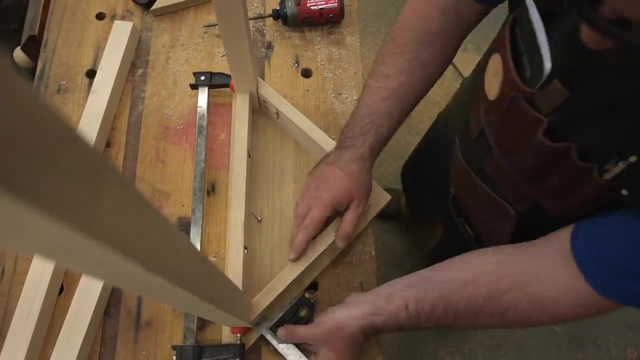 is: do the pocket holes on the inside of the aprons so that way they're not visible from the outside. And we're gonna do pocket holes everywhere the aprons meet the legs and then a few to attach the top. I haven't attached it yet. 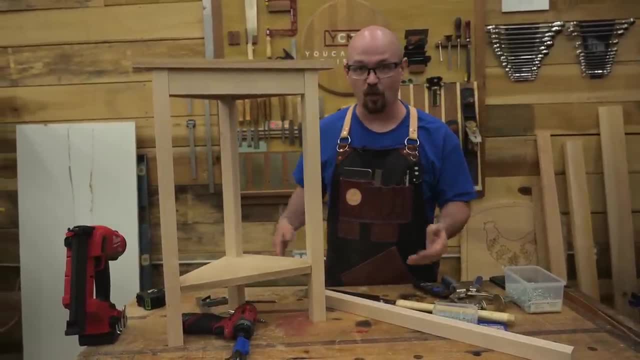 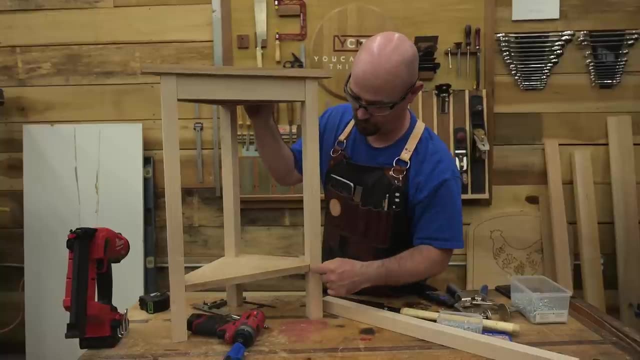 but I got the lower shelf cut out and notched in here. I just kind of wung it and here's the way I did it. It's possible my legs are not perfectly 90 through the top, so I measured where the legs need to be. 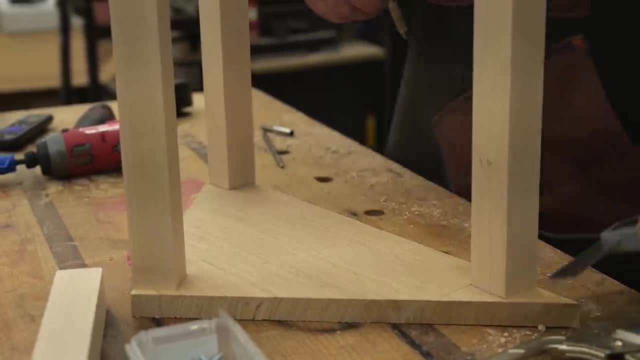 and then I set my shelf down, put the legs on top of it so I can mark the depth for the legs and how the notch need to fit, as well as where the back of it needs to be. So the back leg needed to be cut. 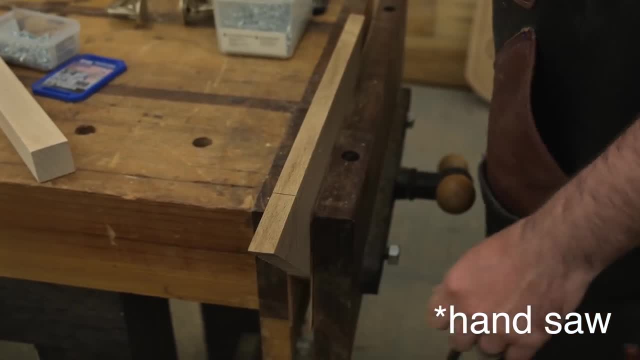 And then, because I wanted these to be fairly precise, cut those out with the circular saw and then just slipped it in here. I literally just stood here wiggling up and down till it looked pretty good. I like this. I think it's six inches. 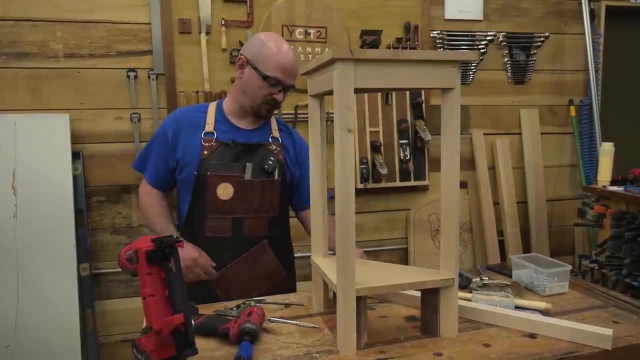 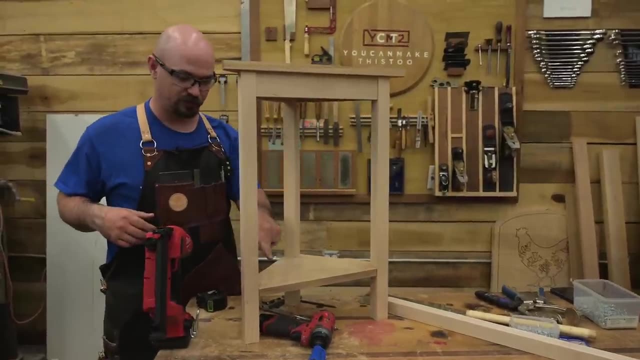 from the bottom to the top, And I cut three little spacer blocks from scrap to hold it, so it's the same on all sides. Now, as far as attaching it goes, I could do some pocket holes on the bottom side. This just really doesn't need that kind of strength. 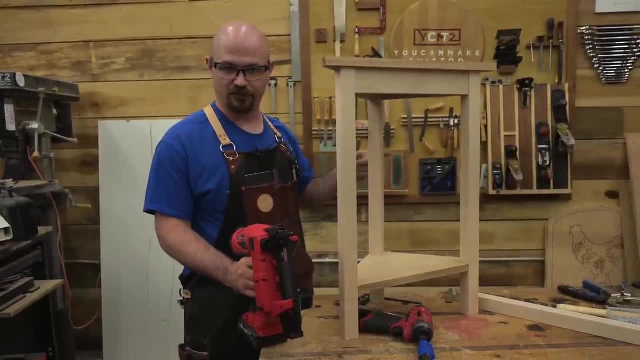 and it's gonna be a pain in the butt because I've got a dull bit for that jig, because a friend has my gun, So I'm gonna do that. It's a good jig right now, So I'm just gonna use some brad nails to pop in here. 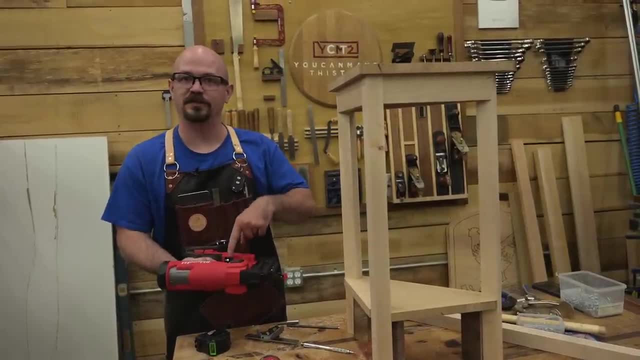 and that'll be just fine. I always forget this stupid thing has a power button. It's like my only cordless tool with a power button, So you don't just put the battery in and go like you've got to turn it on. 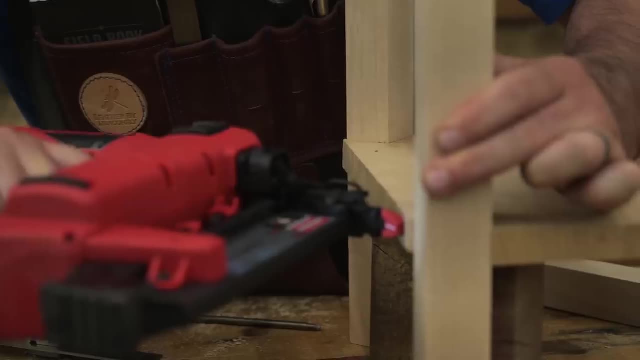 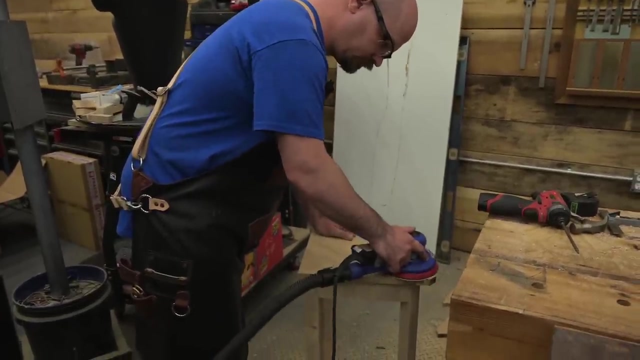 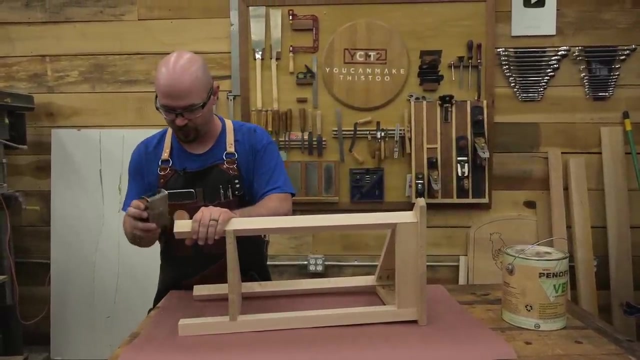 after you have the battery. It's really weird. I broke all the edges with some sandpaper And one very important step on tables is, whenever your legs are, make sure you put a little chamfer or a round over on the bottom. I'm using a plane just because it makes me feel. 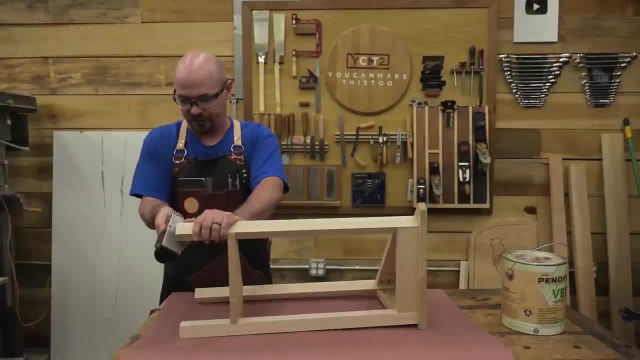 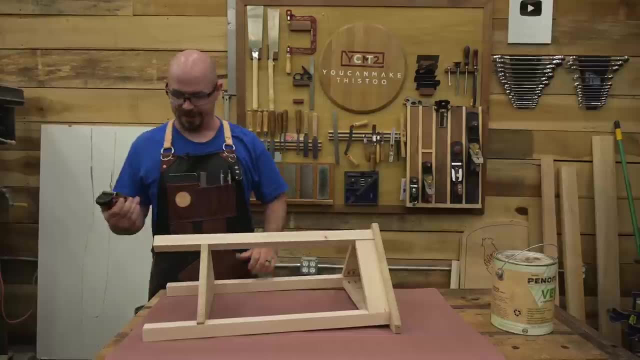 like a real woodworker, and I have one. You can totally do this with sandpaper, though, And the point is, when this gets scooted, drug moved around the floor. if you don't have that and a little pebble. 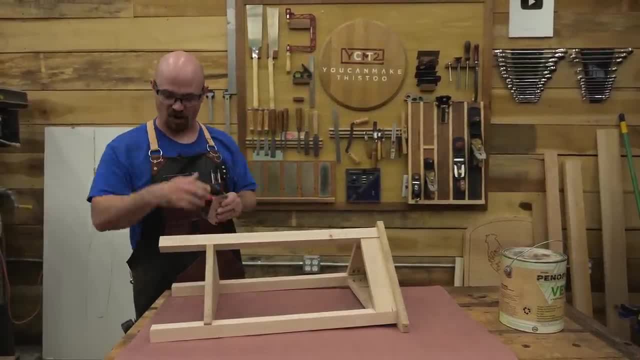 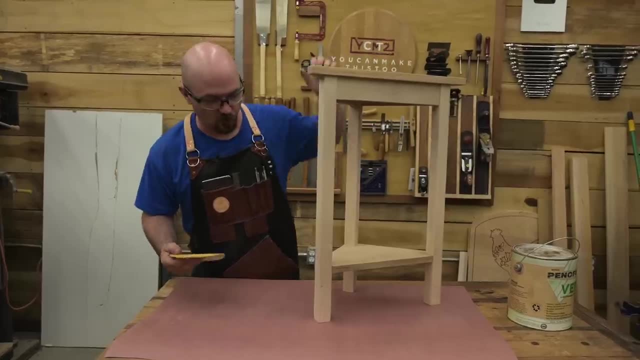 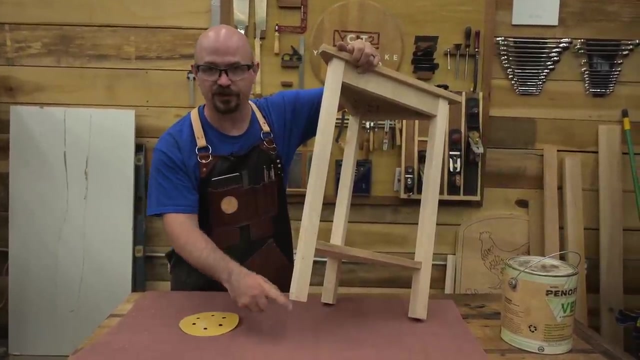 dirt, anything catches it, it can easily grab those fibers and you get a big tear. And by breaking the corner and edge I really mean something this simple. That's done, and all we're doing is taking the sharp edge from being machined and just knocking it down. 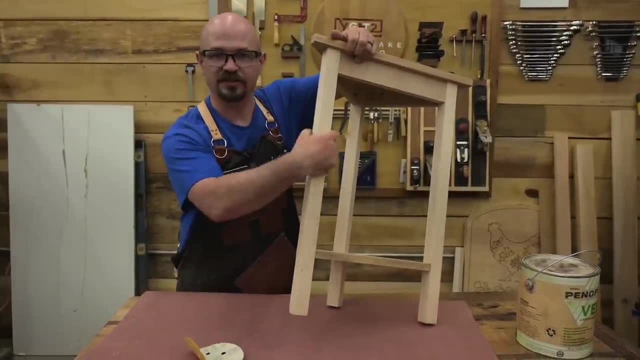 a little bit with sandpaper. This is 180, just so it's not sharp. so when you touch it it's like: oh, that's pleasant. I'm not worried about getting a not paper cut but a wood cut. 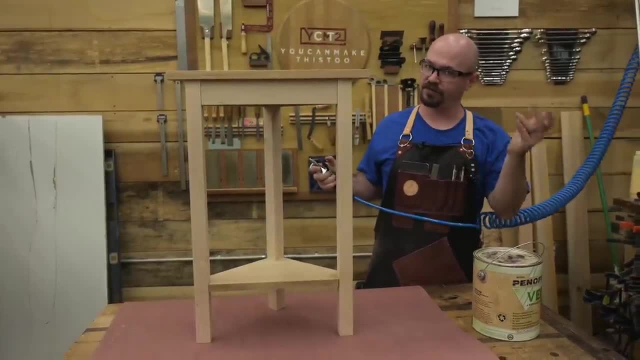 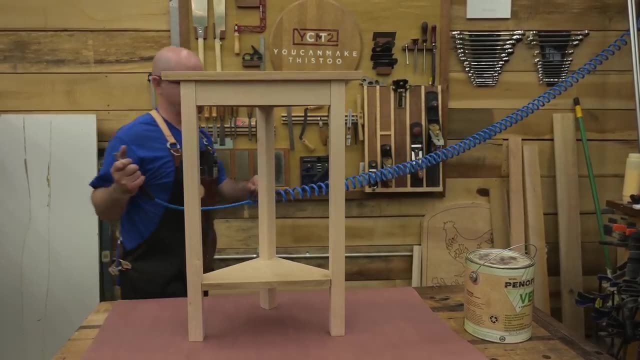 And before we finish, we want to make sure we get all dust off. A damp rag does well, but then you got to let it dry. I've got air, So that's what I like to use All right time to finish. 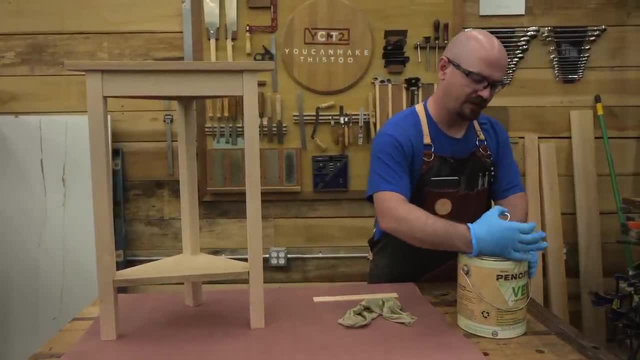 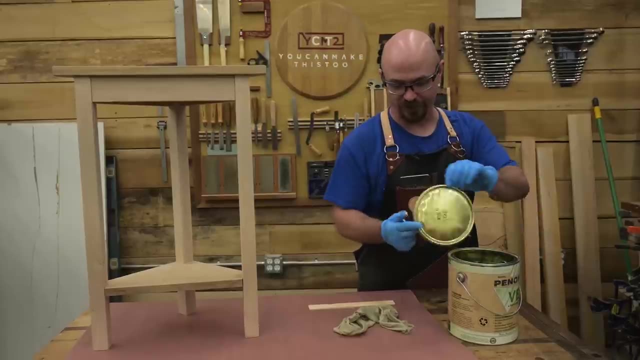 I'm using a not very common product, but I had to order it in a gallon for another project and it'll be fine on this one, so I'm just trying to use it. But you could use any kind of polyurethane walnut oil. 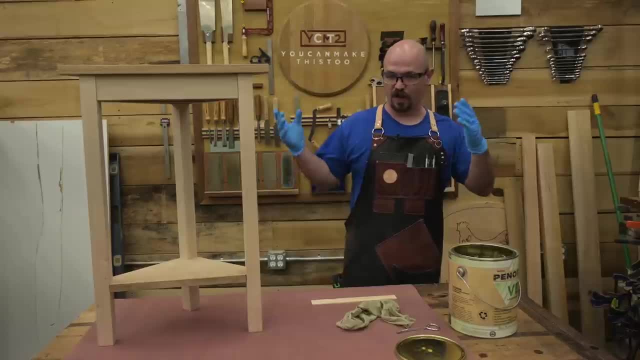 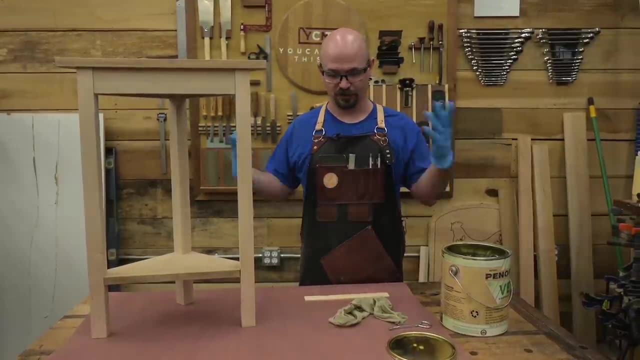 boiled linseed oil, spray, lacquer, beeswax, butcher, block conditioner, whatever you want to finish this with, especially a small utility table is fine. Now, if you're making like a dining table or something that's going to see a lot of use. 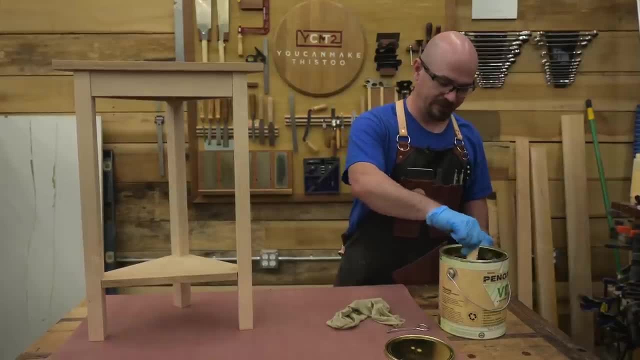 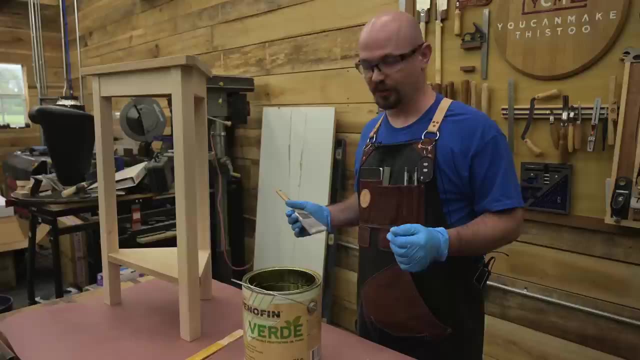 polyurethane is fine, But if you're making like a dining table or something that's going to see a lot of use, polyurethane would definitely be a good route, Just like sanding and wood filling. I have an in-depth video on finishing. 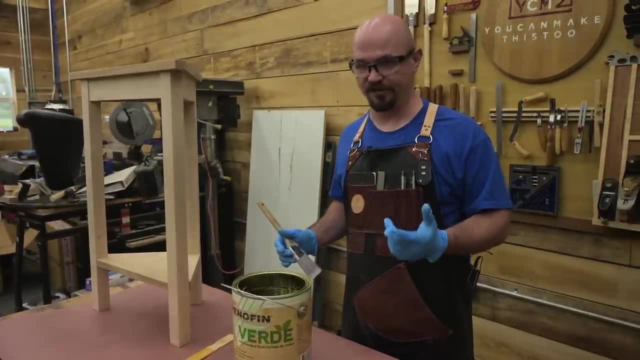 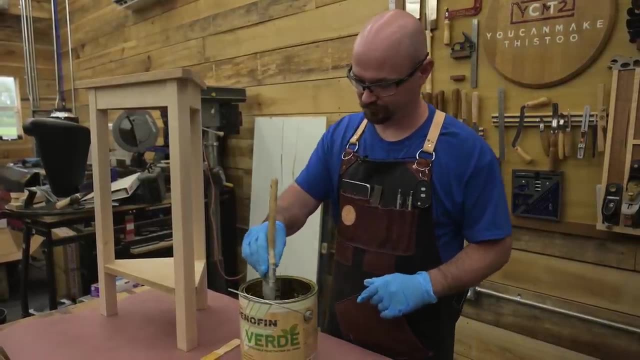 The real meat of it is basically read the directions on the label. Manufacturers want you to have a good experience, and those are best practices. Follow the best practices. You'll probably get the best results While you get to check out the beautiful oiling shots. 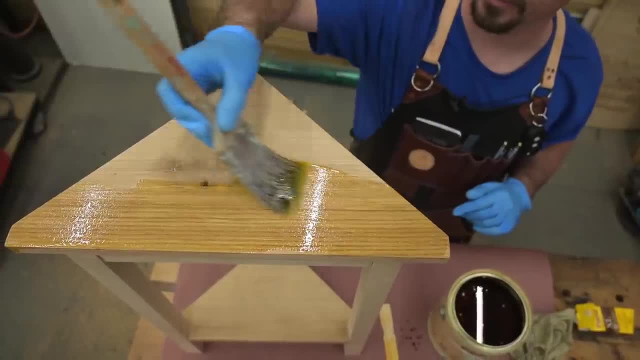 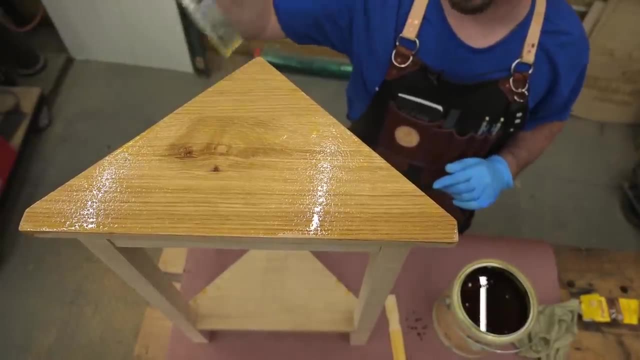 I'm going to talk about possibly the most important step, which is coming up very soon, And that's when we're done And we take this inside and it's visible to the public. Now this is something that plagues beginners and professionals alike. 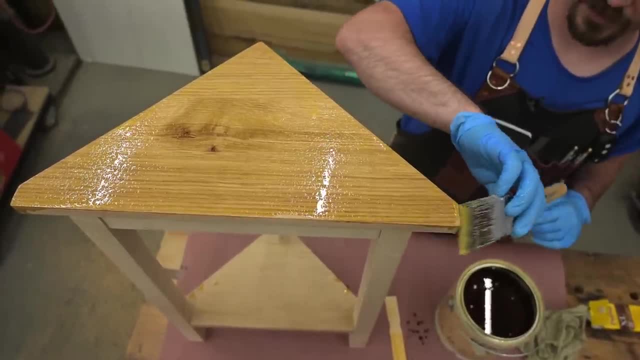 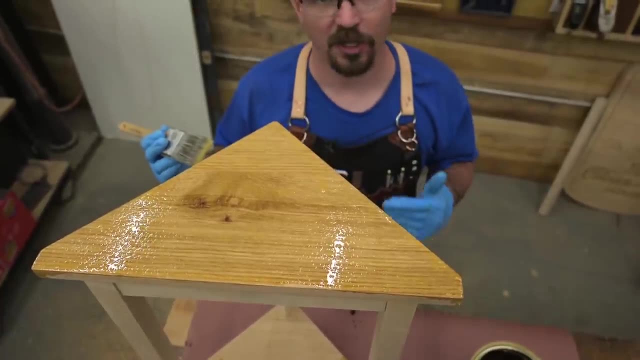 When someone sees your work that's finished, they're going to be very tempted to correctly and appropriately say: whoa, that's beautiful, That's great, That's amazing. You did such a great job. And your intuition will tell you to say: 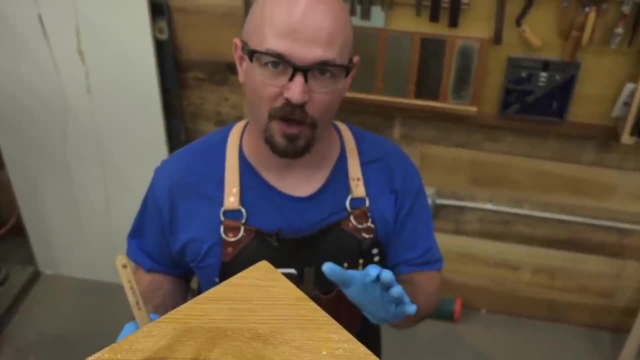 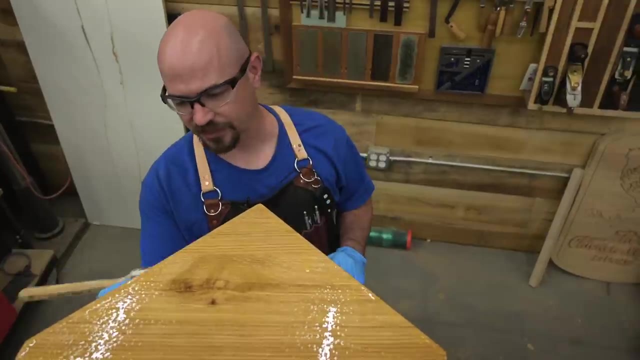 hold on. I've got to point out every single flaw. You falsely complimented me, And that is not acceptable. How dare you compliment something that is not perfect? Let me correct you. Actually, that's totally wrong. What you should say- this might be tough is: thank you. 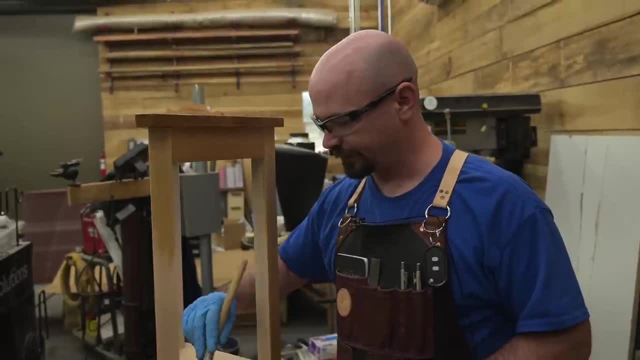 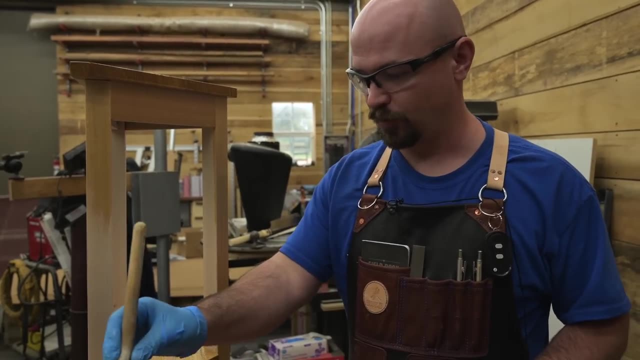 They already knew it wasn't perfect, Believe it or not. The other thing is they don't care, because nothing's perfect and they don't expect perfection. What is amazing and is perfect and is beautiful, regardless of whatever flaws are in your piece. 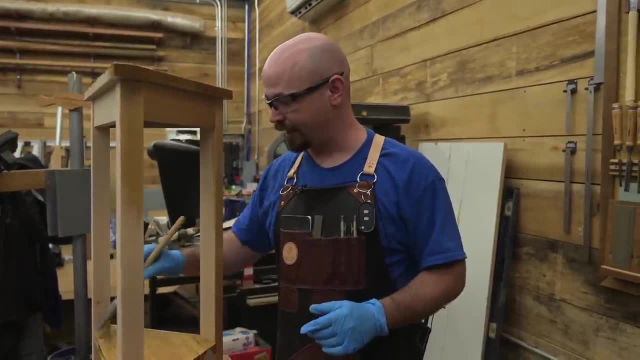 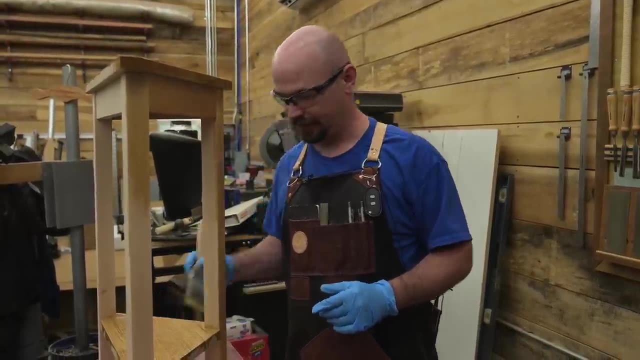 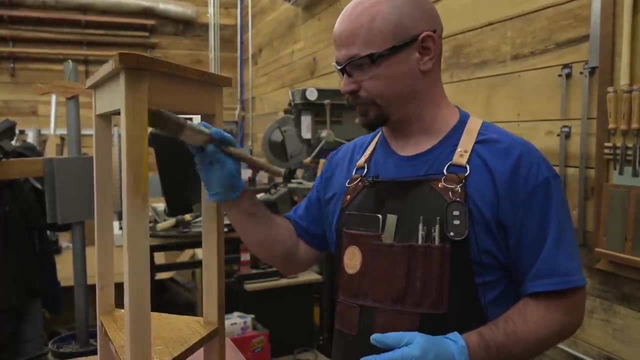 just like the flaws I have and you have and everyone has, is that you took What was raw material- just stuff scrap that might typically be seen as basically just a firewood or landfill- and brought it to life and gave it purpose. 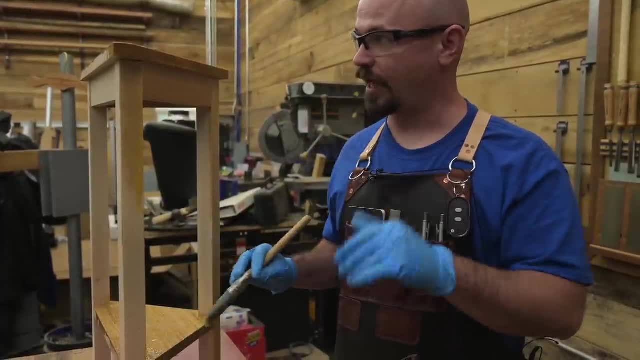 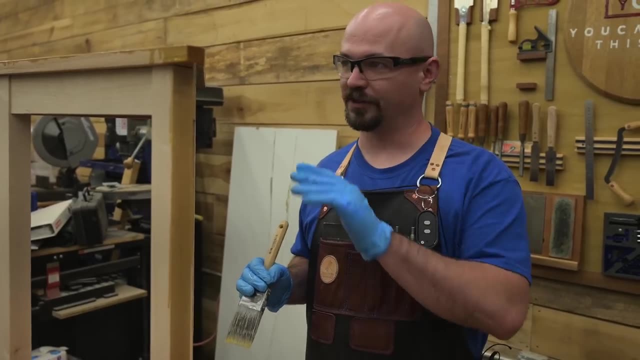 All these pieces were just junk outside, eventually going to rot and probably get burned if they didn't get a purpose Promptly enough. it's now a table that's going to serve a use and purpose in our house. It's a slight problem for us. 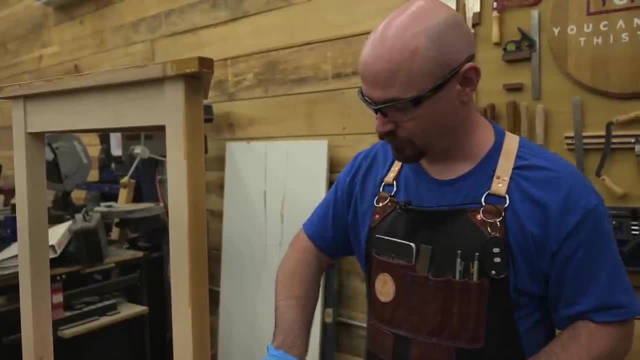 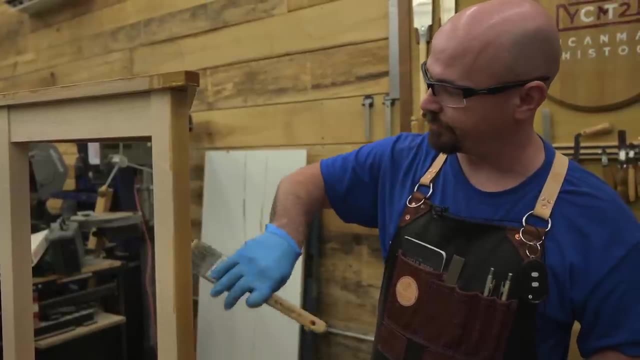 That is beautiful. That is really cool. That doesn't change with any gaps in joinery that are present, or if the finish isn't completely even, or if there's a spot that I didn't perfectly sand, that I missed. well enough, It's still amazing. 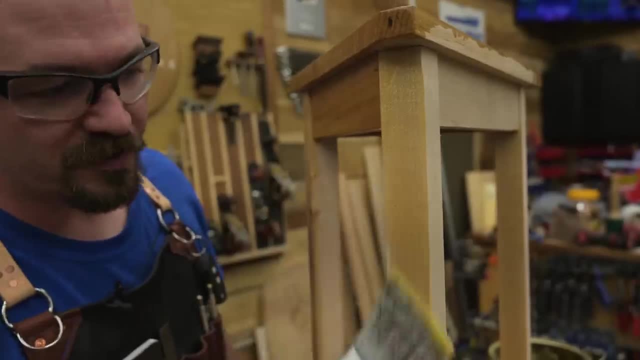 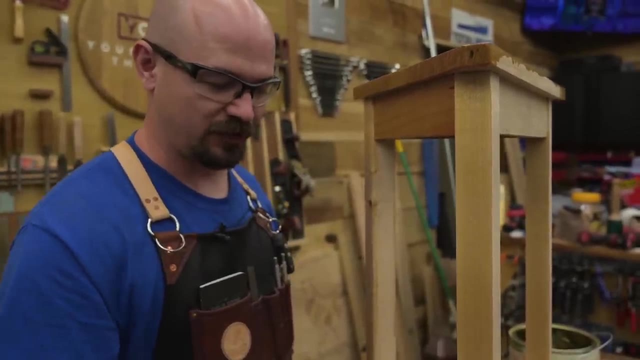 So you say thank you, You just say thank you. That's all you have to say, Because if you've ever complimented somebody and they come back with, oh you're wrong, Look at my acne. or the hairdresser didn't do a great job. 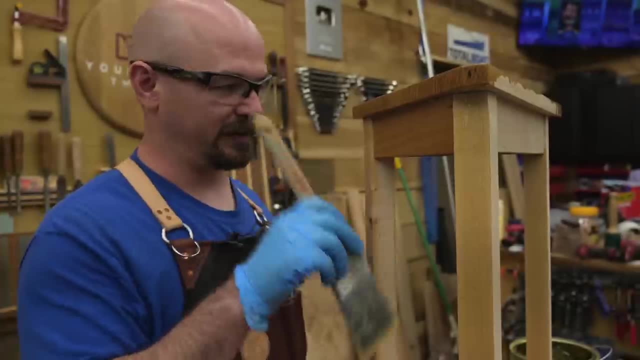 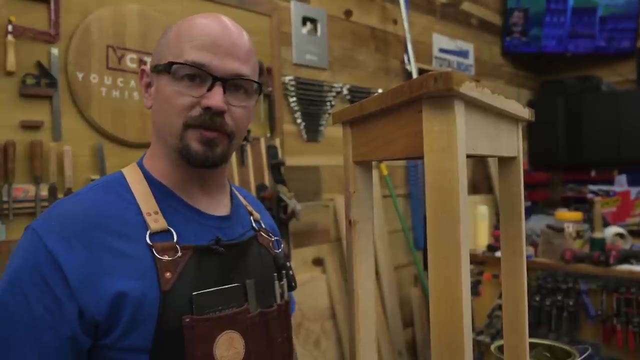 But look at this crack and look at that gap and how these two things aren't even and blah, blah blah. If you've ever had someone do that to you, you instantly go from thinking. I'm really impressed by what's happening here. 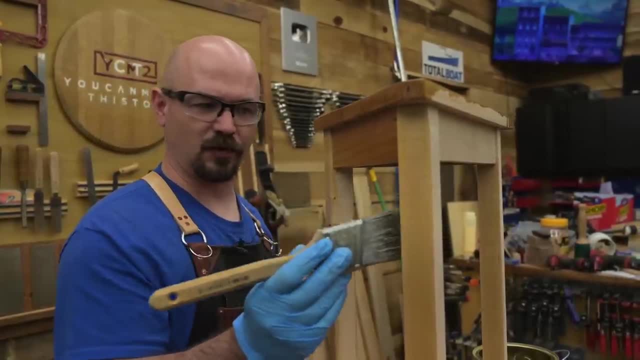 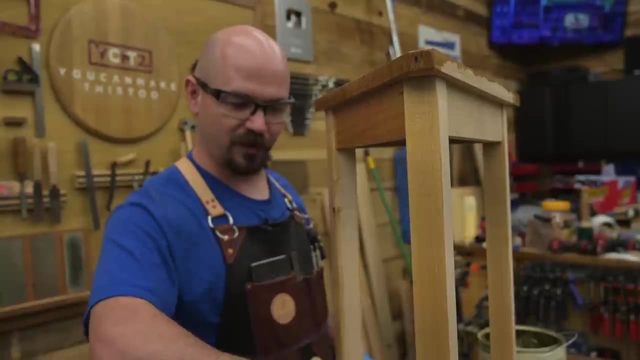 to. I don't know what to say. This just got really awkward. You know what I lied? It's total crap. You should never try this again. Like, what are you looking for? It's not about you, Think about someone paying you a compliment. 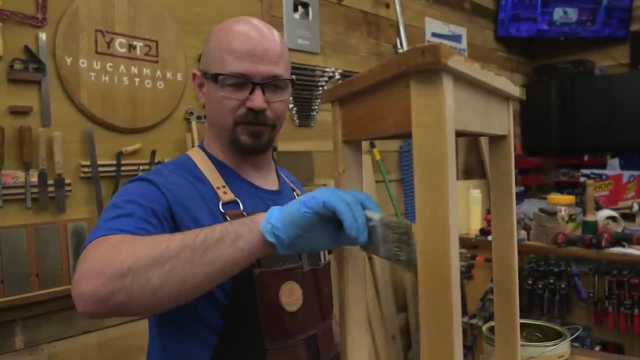 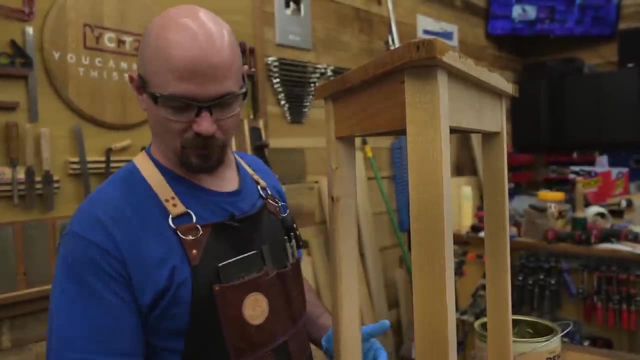 and they just want to hear thank you. and everything they're saying is true, because it is beautiful that you took junk and then brought it to life And gave it a purpose. You made something exist that didn't exist before And similarly right. 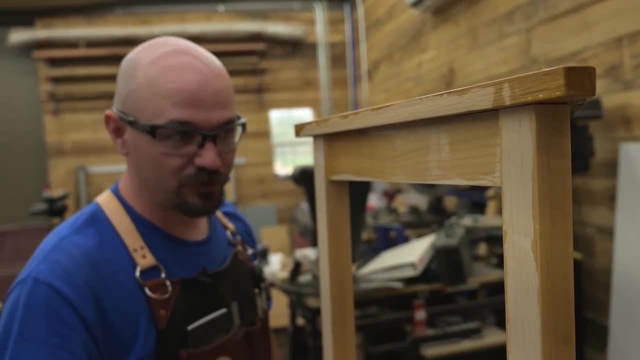 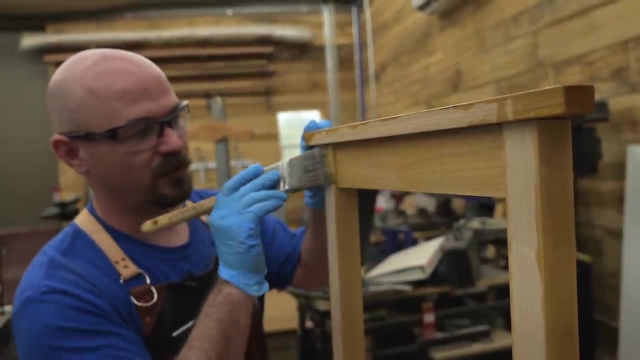 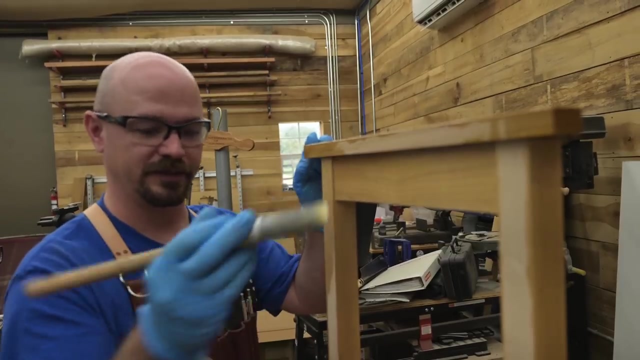 If you have someone in your life who just doesn't know how to take a compliment, instead of trying to force them to there is a better way- especially if they make stuff- to pay a compliment that they can't crack down, And that's just to simply give it differently. 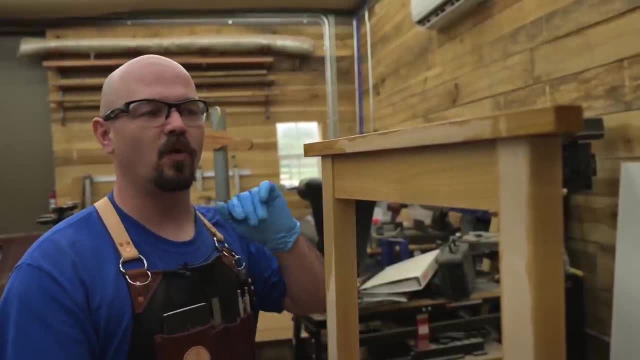 So, instead of when you see something saying, oh you look great today or that's a great piece, that's beautiful, that's amazing, whatever where they're going to be like, oh, let me show you all the flaws, right. 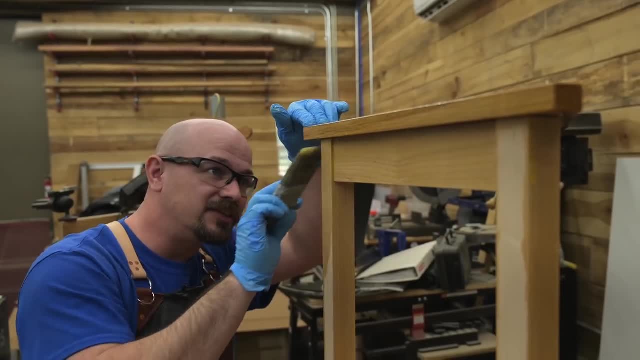 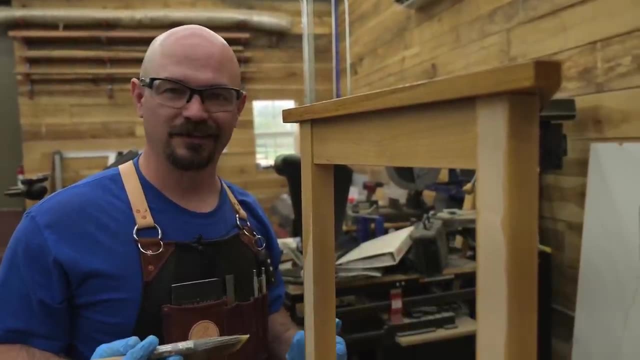 Especially if they made something. The way you can pay a compliment that they can't shut down is to say: I'm so blown away. you took what I would see as junk and gave it purpose. That's so cool. In a second I'll show you what this looks like.